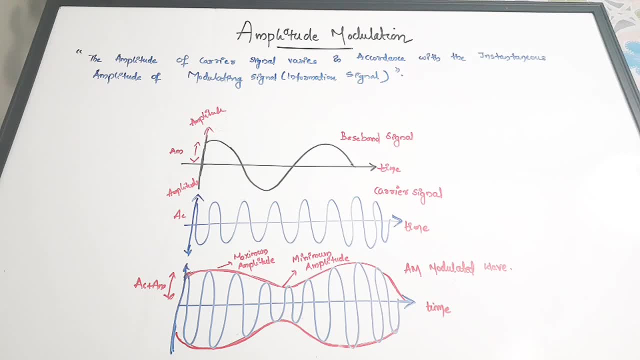 modulation, what is actually happening in it, how the carrier wave is getting modulated, what is the concept, and also we will be seeing all the major areas like the bandwidth equation, the actual signal equation for the air modulated wave, and also we will be seeing the equation. 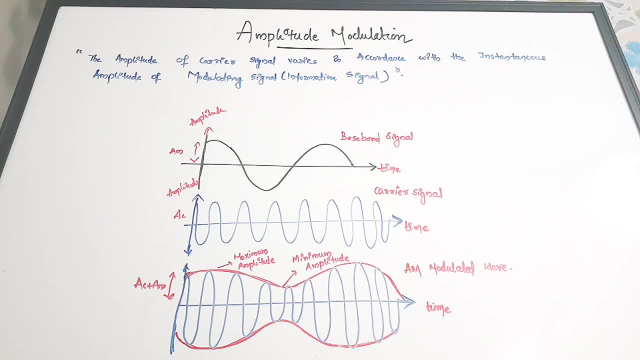 for modulation index and the spectrum also. Okay, so amplitude modulation means here we are actually going to modulate the amplitude of the carrier wave in accordance with the instantaneous amplitude of the modulating signal. Okay, so you should be knowing that there are two signals here. One is the information signal. You can call it either information, 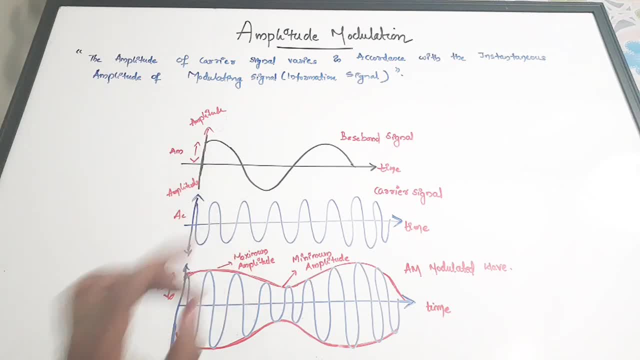 signal or baseband signal or modulating signal. Okay, you can use any of the three words. Generally we use these three terms. In some textbooks you can see baseband signal. In some textbooks it will be modulating signal. In some textbooks it will be written as information. 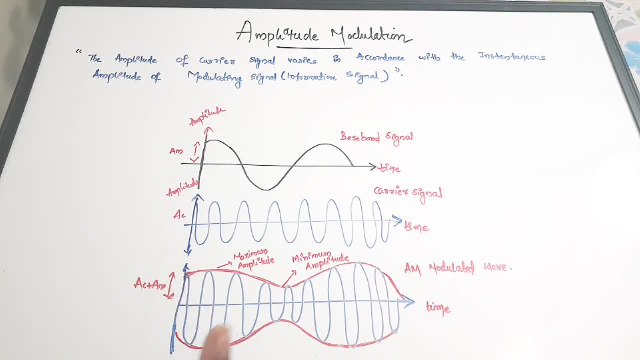 signal. Anyway, the three things is indicating one signal, which is our information signal. Okay, so this information signal, we know that it is of lower frequency, But we have explained in the modulation that is need for modulation video that these low frequency 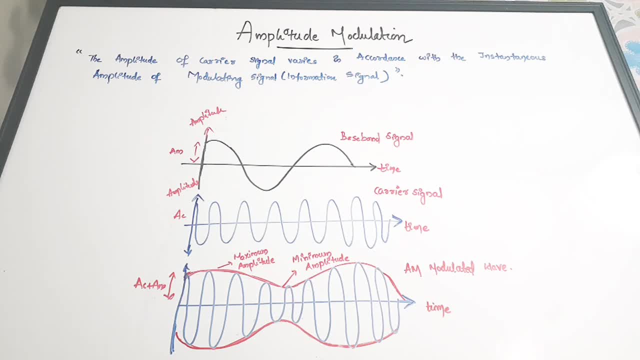 signals get attenuated or cannot be sent. So we use a high frequency carrier wave. So this carrier wave, you see, it is actually carrying zero information or it is having no information, but it is just a carrier, It is just a carrier of the wave. 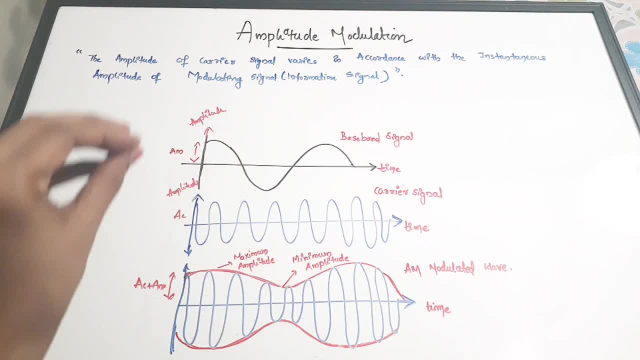 Wave. That is, it is just a carrier of our actual signal, which is our information signal or the baseband signal. Okay, so that is why we call this signal as carrier signal. Okay, so this is our actual information signal or the baseband signal. This is just a carrier. 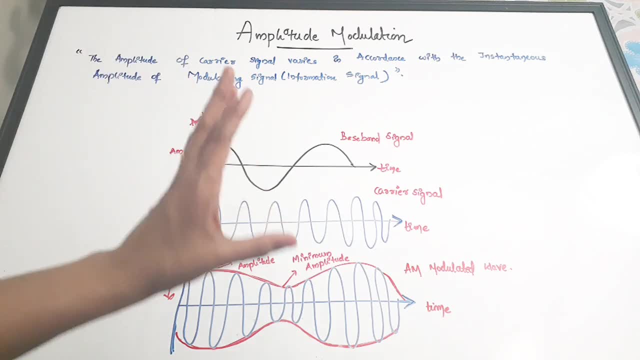 signal which is not having any information, And we are going to modulate the amplitude of this signal, which is the carrier signal, in accordance with the instantaneous amplitude of our information signal. So this black color represents the information signal, or the baseband signal, In accordance with the instantaneous amplitude of this signal we are 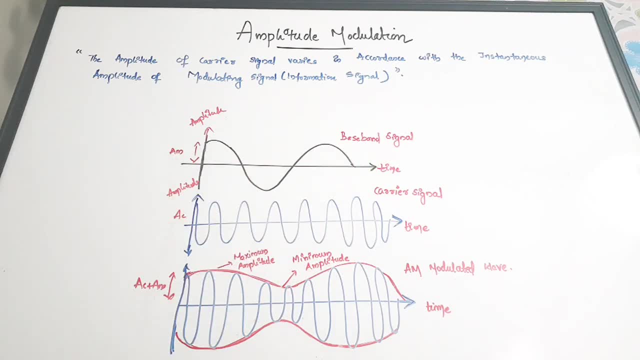 going to modulate the amplitude of this carrier wave and we will be getting a waveform like this and this process is called amplitude modulation. I hope you have got the idea of amplitude modulation. So the amplitude modulation I will say as a definition, So the amplitude of the 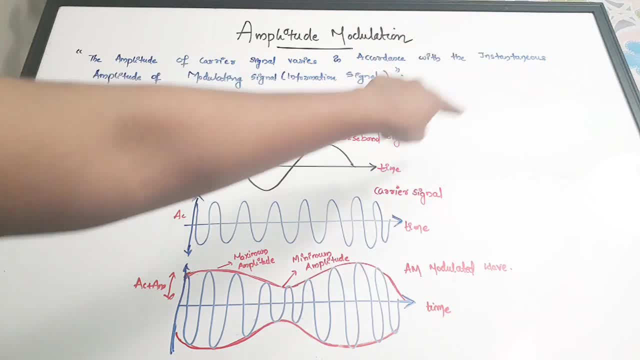 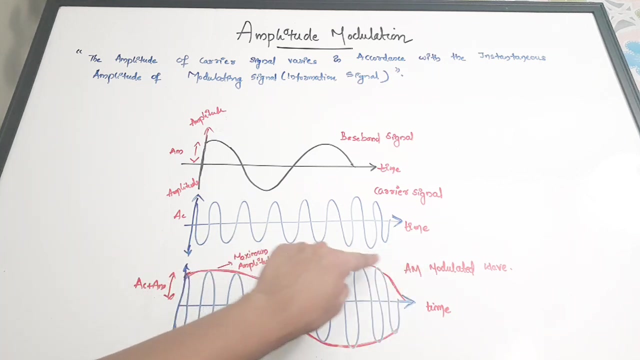 carrier. signal varies in accordance with the instantaneous amplitude of the modulating signal. So this is the carrier whose amplitude is getting modulated in accordance with the instantaneous amplitude of the modulating signal or information signal or baseband signal. So we will be getting a waveform like this. You can see that here the carrier. earlier it had a. 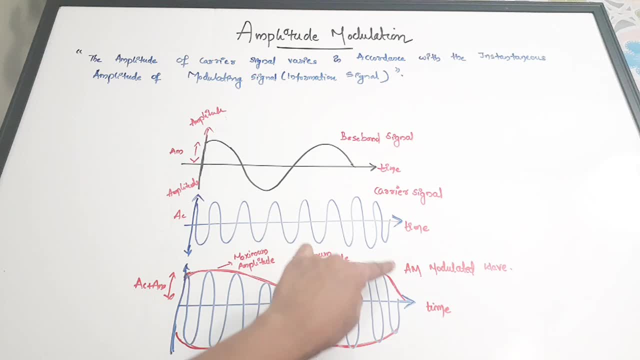 single amplitude, right, but here the amplitude is getting modulated. So this is the carrier whose amplitude is getting varied in accordance with our original information signal. So there is a red color line drawn over the carrier wave, or the outer edges of the carrier wave, and that is. 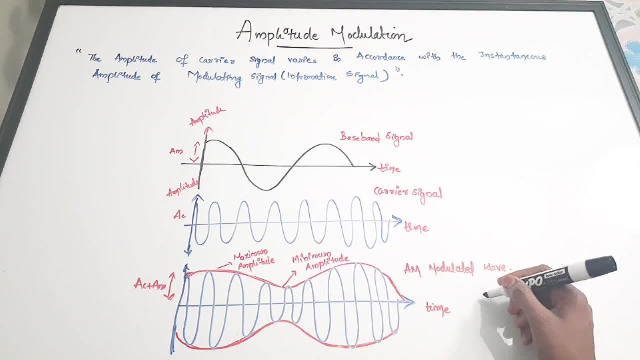 called a envelope. This term is also very important because when we study the detectors of AM modulated waves, we will study a detector called envelope detector. So this red colored line which is the outer edges of the AM modulated wave is called envelope. So this is the envelope and this 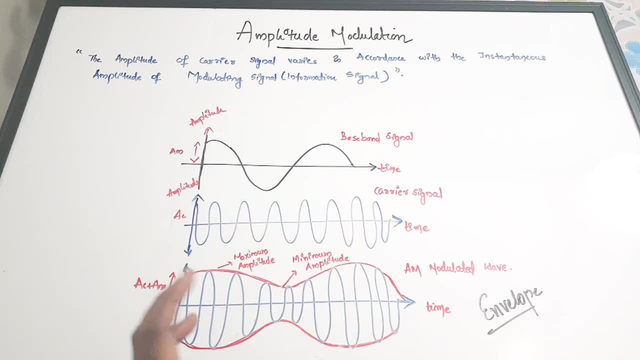 envelope will help us to recover our original baseband signal easily. So this envelope help us to recover our original information signal easily from the modulated wave. So this is the modulated wave, which is the AM modulated wave. So this AM modulated wave is nothing but the AM modulated wave. 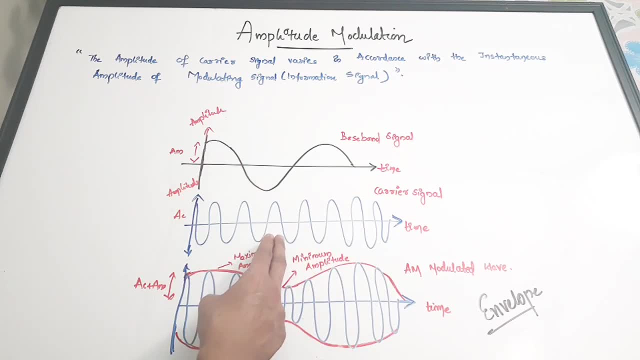 Amplitude modulated version of our carrier signal. So the carrier signal has undergone some amplitude modulation and we got a waveform like this. This is called our AM modulated wave and this AM modulated wave in that there is a maximum amplitude area and also there is a minimum amplitude. 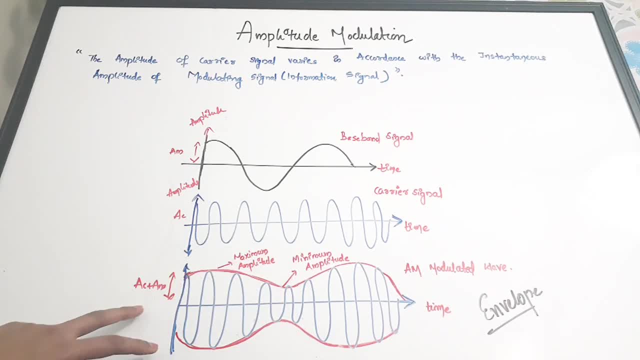 area. So this total maximum value will be equal to AC plus AM. You should be knowing all these things. I hope you understood that. the figure one, that is the top figure, is indicating the message signal or the information signal or the baseband signal. Figure two: this one is indicating the carrier wave. 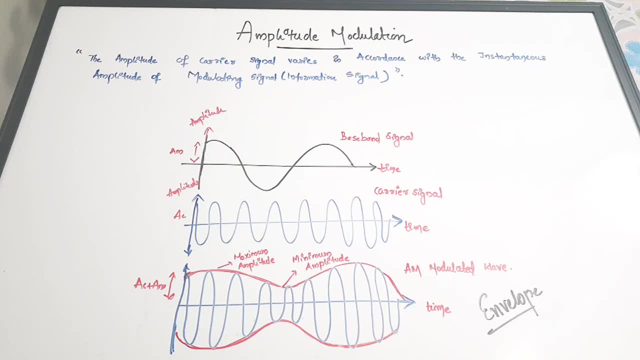 it is a high frequency wave and it is carrying no information. and the figure three is representing the corresponding AM modulated wave. Okay, and another important thing you should be knowing that the red colored line drawn through the outer edges of the AM modulated wave is called AM modulated. 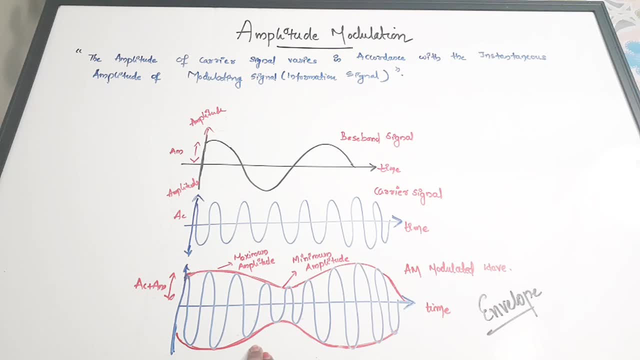 wave. The outer edges of the modulated wave is called an envelope. So this it is actually same as that of the message signal. It is just like that of the message signal and this line will help us to extract or to recover our original information signal. Okay, so that is the concept of a AM modulation. Now let's 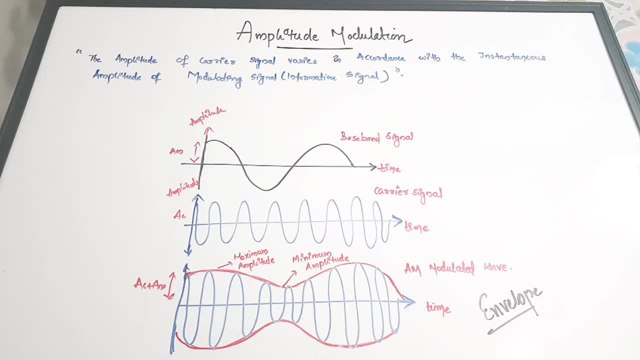 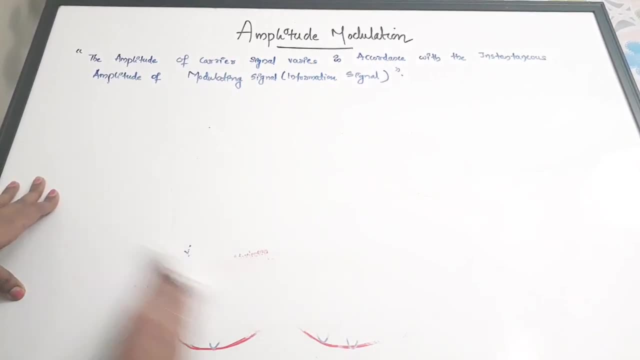 see how can we give the mathematical representation of a AM wave. Okay, now let us see in the expression forms or the mathematical representations. Okay, so let's see. Now we are going to write the time domain equations for all the waveforms. First, the waveform we have is modulating signal, or our. 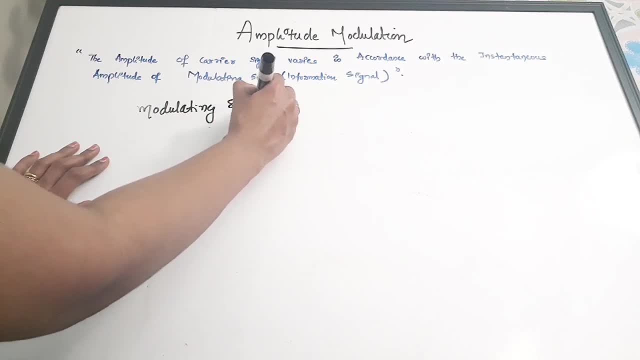 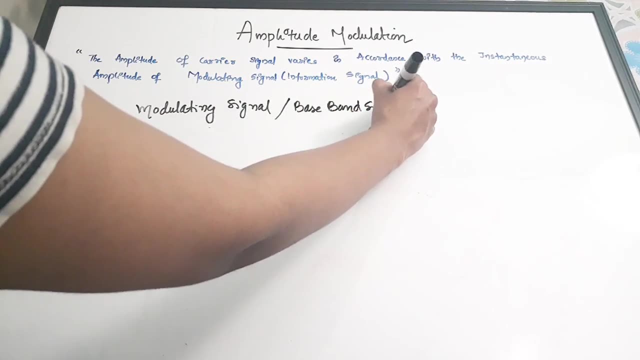 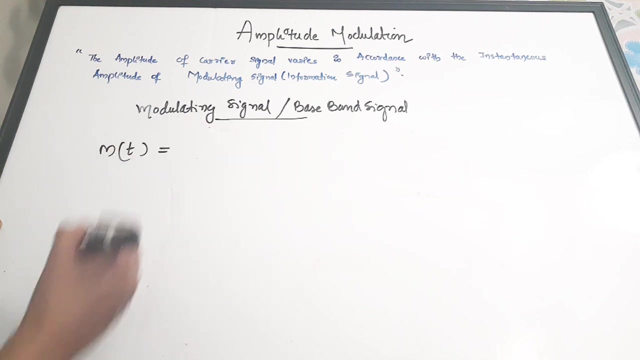 our baseband signal. you can say baseband signal or modulating signal. Both terms you can use are modulating signal and you are going to represent, or I am going to represent it using the letter or variable m of t. m of t is equal to AM, cos 2, pi, fmt, So it is a sinusoid cosine waveform. 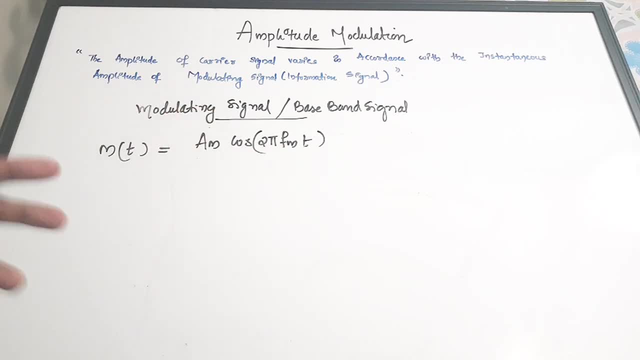 Okay, so m of t is the modulating signal, or our information signal, and it is represented as AM, cos 2, pi, fmt. and the carrier signal I am going to represent is carrier C of t is equal to AC into cos 2, pi f C of t. So this is the carrier waveform representation. 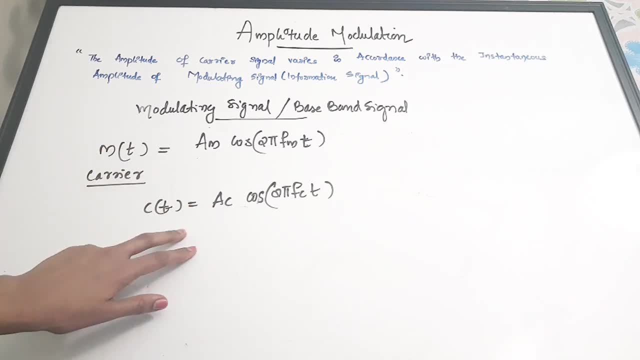 Now, if this is the modulating signal and this is the carrier, now let us see what all terms are present inside the equations or the expressions. Now, AM, what is AM? AM is the amplitude of the modulating signal. Okay, write it here. AM is the. 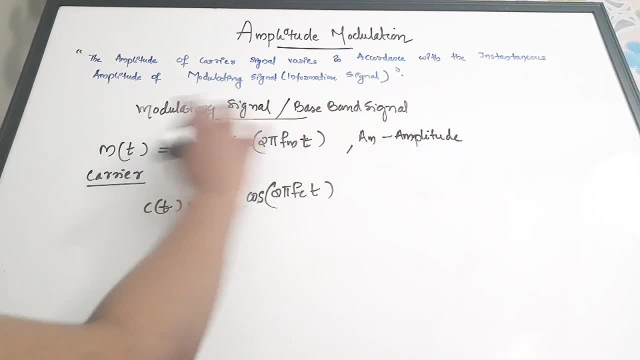 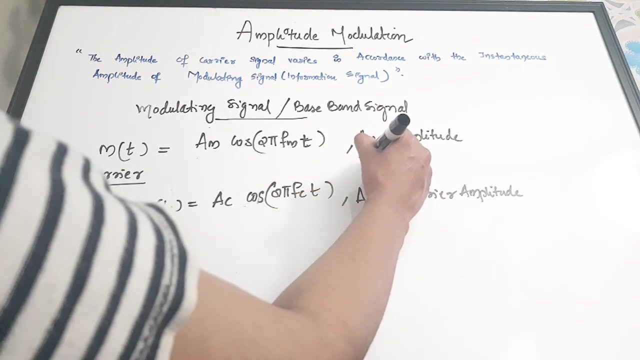 amplitude of the modulating signal or the baseband signal. Now, AC is the amplitude of the carrier: Carrier amplitude. Okay, so that is AC. Next, there is another two terms, which is fm and fc. What is fm? fm is the frequency of the modulating signal. Okay, fm is the frequency of 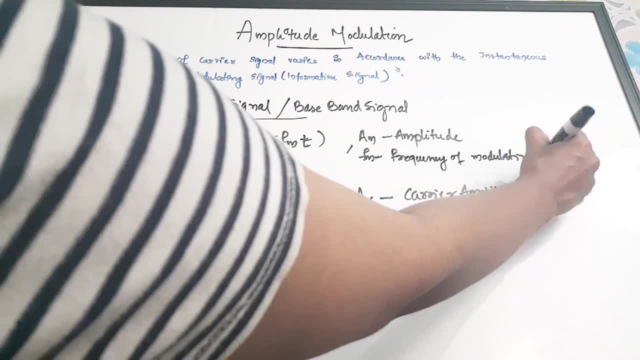 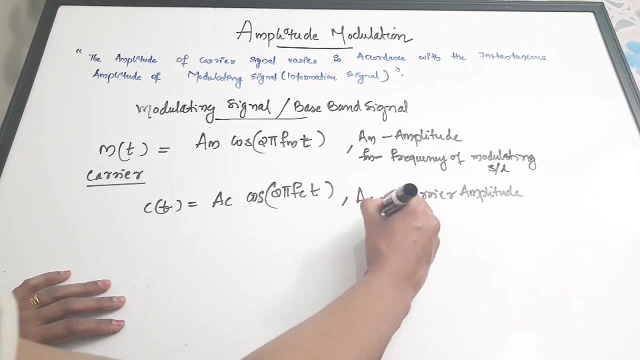 modulating signal. Okay, then here fc will be the frequency of the carrier, fc is the carrier frequency. Okay, so we have discussed what is AM, what is AC, what is fm and what is fc. So these two expressions are the expressions for our modulating signal and the carrier signal. 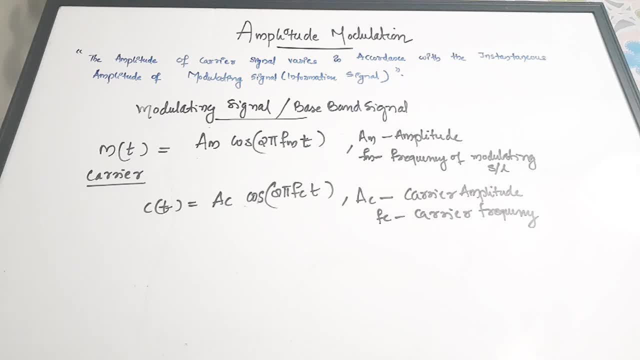 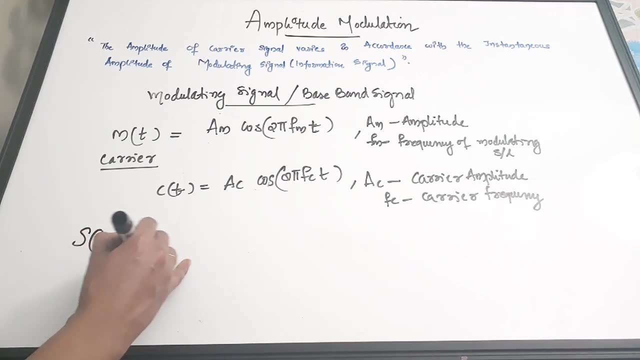 Now, if this is modulating and the carrier waveform, modulated waveform- will have an expression like this. So I am going to write the expression directly: s of t is equal to ac plus am, cos, 2, pi, fm, t. this much will be the amplitude portion. 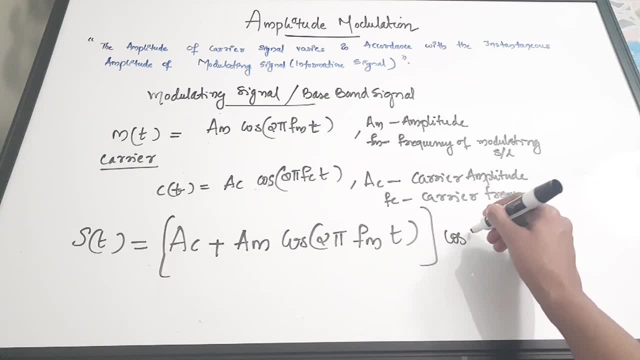 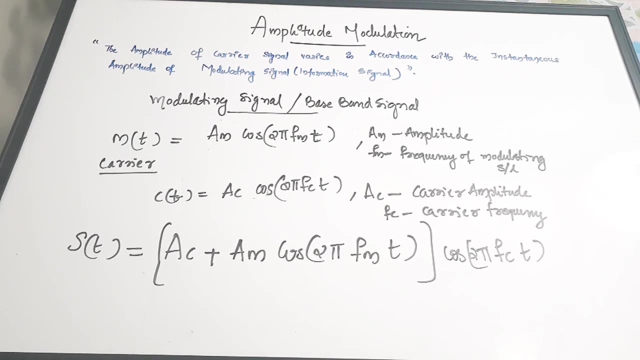 into the cosine form, that is, cos 2, pi, fc of t. So here you can see that there is a cosine term with a frequency, fc. So the frequency is the frequency of your carrier waveform itself. So if you compare this modulated waveforms equation with the two equations above, you can: 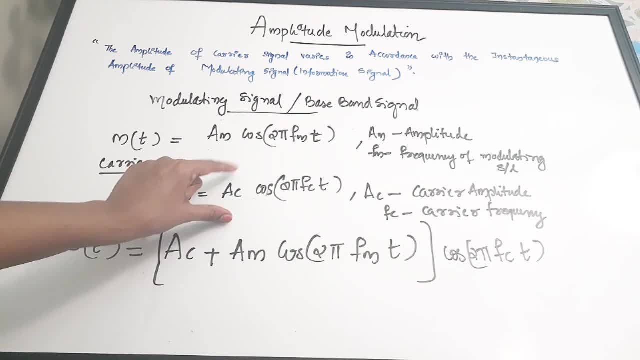 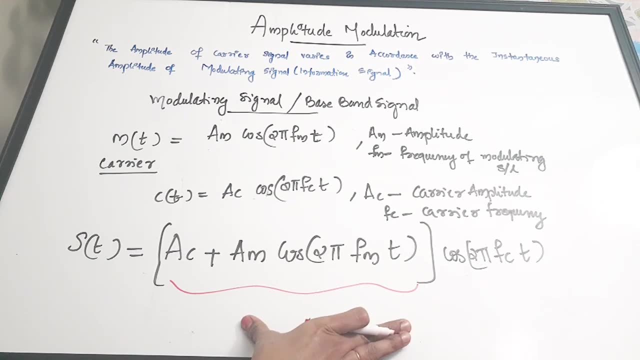 see that this portion is corresponding to the amplitude. So this is the, this much. that is, this much is the amplitude of your am modulated wave and this represents the frequency or the frequency part. yeah, So this is the frequency which is equal to the carrier frequency. So from this expression, it 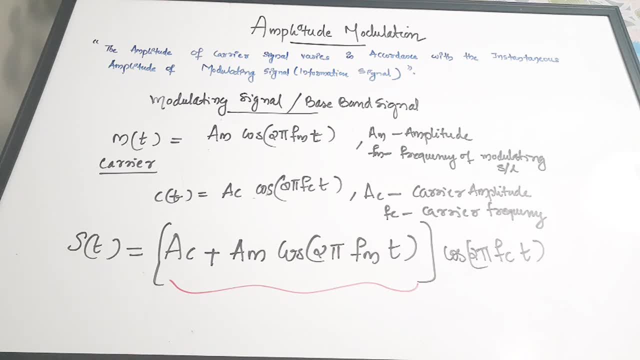 is clear that the waveform there is our am modulated waveform, So this is the expression for am modulated wave, right? So for a am modulated wave it will be having the frequency as same as that of the carrier, but the amplitude will get modulated in accordance with the 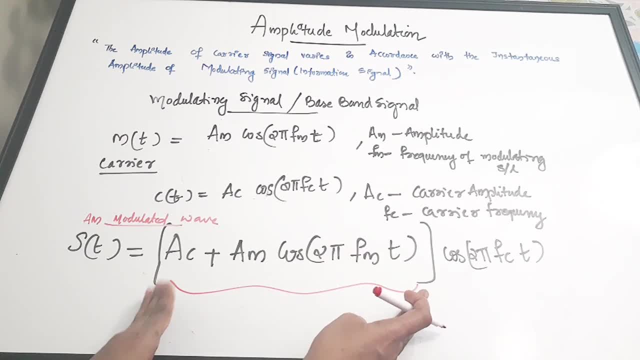 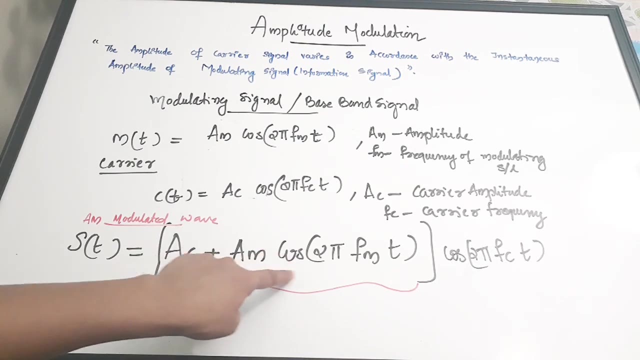 modulating signal. yeah, So this much portion is representing the amplitude and this portion represents the frequency. So this portion, you can see that there is a ac and also, in addition to that, there is one term coming right: am, cos 2, pi, fm, t. So this is nothing but your message: signal, right? this is your. 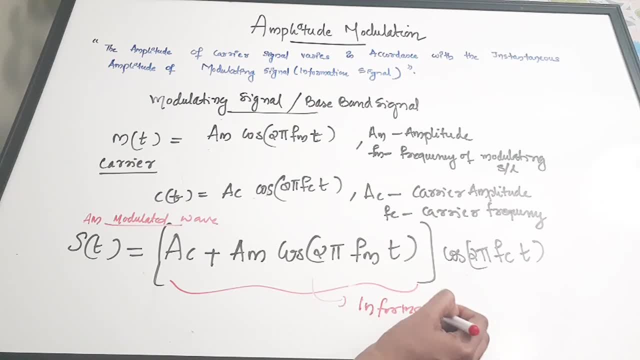 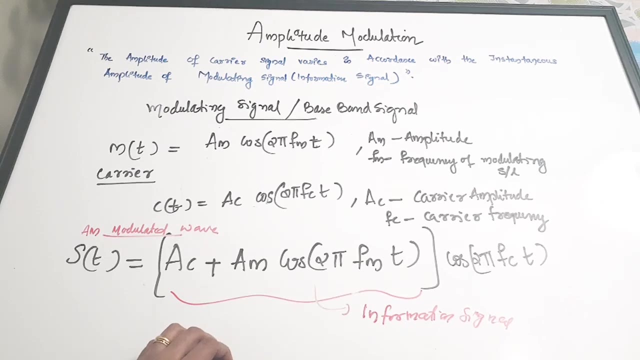 message signal or your information signal. right, so the information signal is getting added to which part? it is actually getting added to the amplitude part. okay, so the frequency will be same as that of the carrier waveform, but the amplitude part will get modulated in accordance with your information signal. that is the concept, okay. 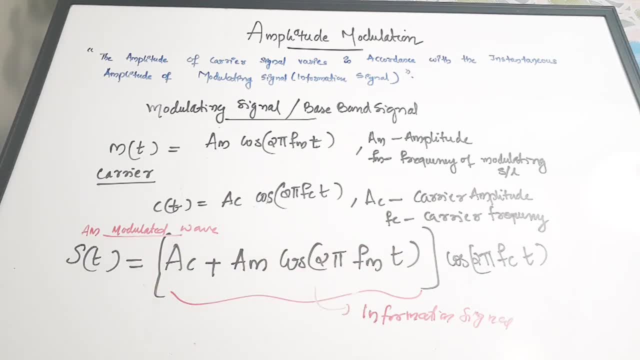 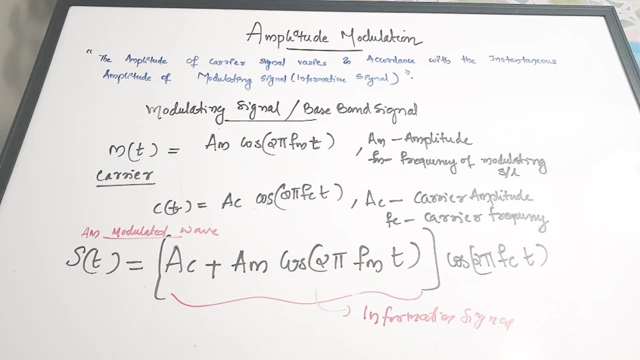 so this is the equation for your am modulated wave. that is ac plus am cos 2 pi fmt into the into cos 2 pi fct. okay, so this is the expression for your am modulated wave, okay. next we are going to see a very important concept, which is called modulating index, because if you are preparing 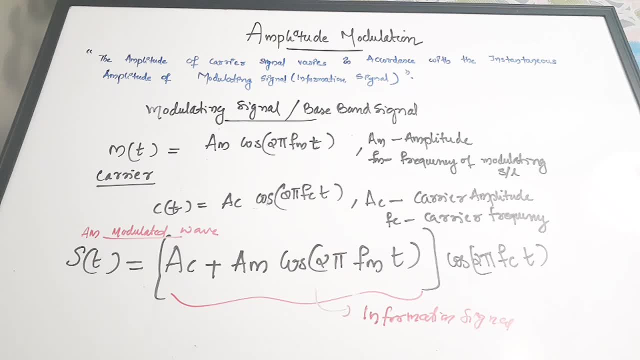 for any competitive examinations this term. this modulating index is very important because you cannot find a question paper without having this term. okay, so let's see about modulating index. i hope you understood this much, okay. next we are going to again see the expression for your am modulated wave, that is, ac plus am, cos, 2, pi, fmt into the. 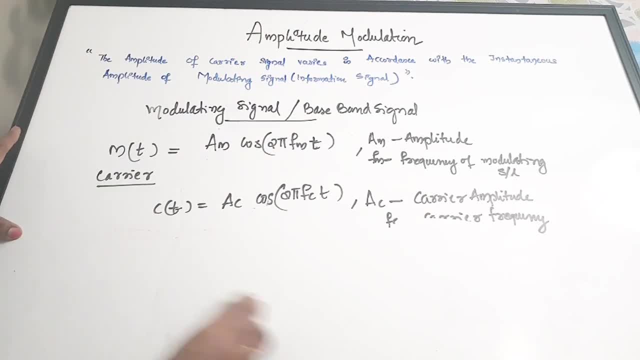 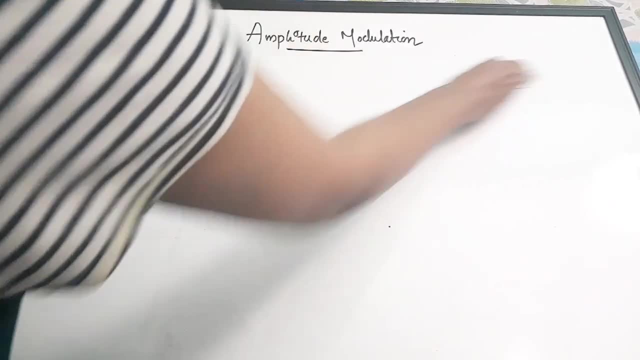 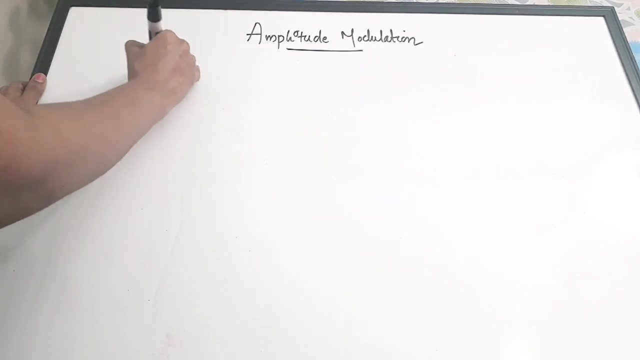 same equation, but i'm going to remove it from the board as of now. okay, we'll write it once again, no worry. so definition also i'm going to remove. next we are going to see the concept of modulating index. okay, now, if you don't know, modulating index, it is the degree with which 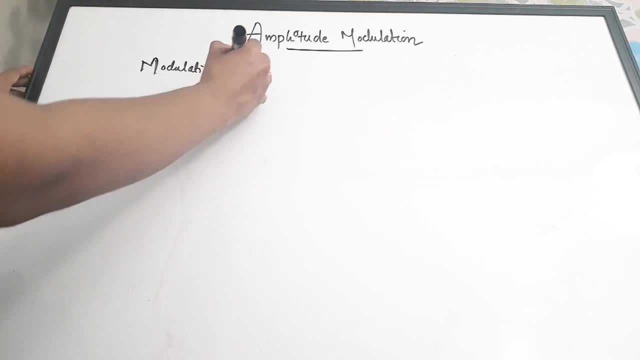 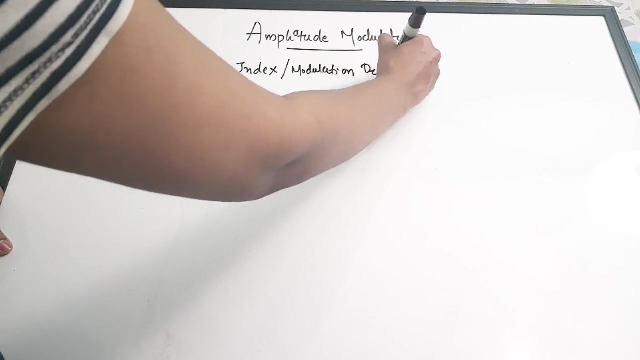 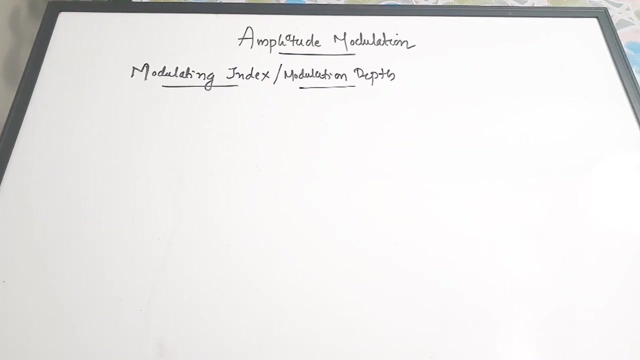 actually the modulation is happening, modulating index. or you say it is modulating index, or you sometimes say it is modulation depth. okay, that is also used. modulation depth: it is the degree to which your carrier is getting modulated. we know that here see, our carrier waveform is actually getting modulated right, we are just using our information signal to modulate. 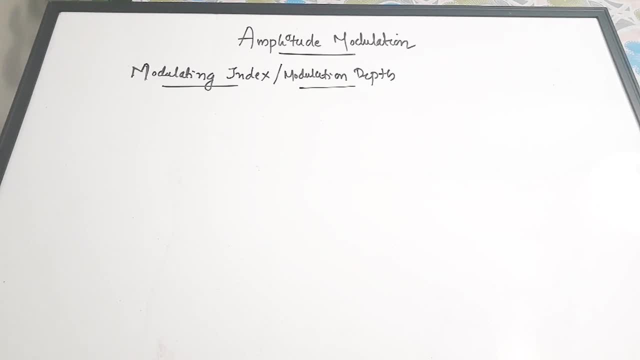 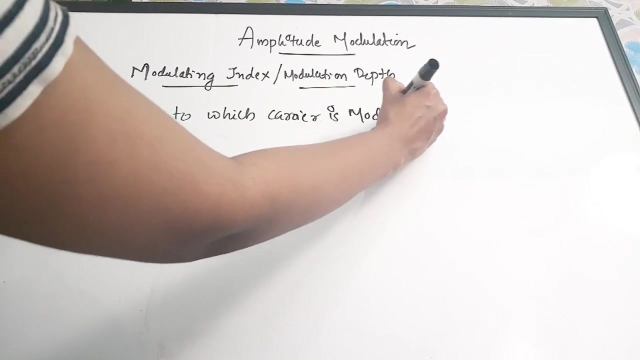 the carrier waveform. so which waveform is actually getting modulated? carrier waveform is getting modulated. so modulation index is the level to which the signal, that is the carrier signal, is getting modulated. okay, that is the level to which the carrier is modulated. is called modulation index. 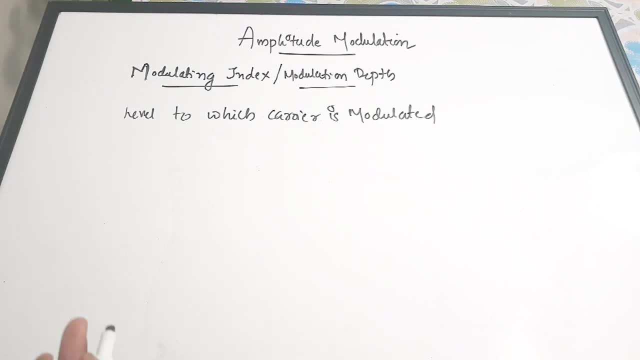 okay, this is a very simple definition. now, if you see the expression of am modulated wave, how can you define modulation index? let us see, okay. okay, so the expression for the am modulated way we have written s, s of t is equal to. we're going to write the. 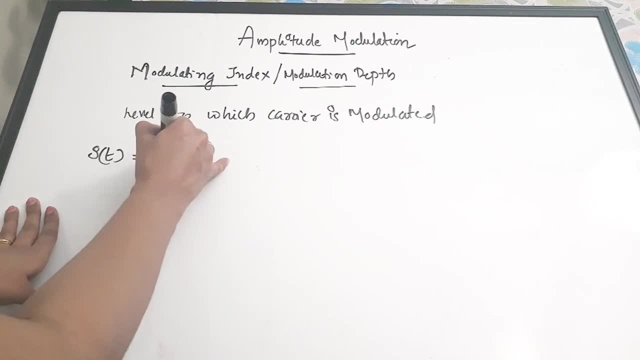 equation which we have written just now, that is a s s of t. we have called the air modulated wave that is equal to ac plus am, cos 2 pi fmt into cos 2 pi fct, right. so we have modulated a ledges which is considered as ay produced mixed model which is attached to m c, not aI. 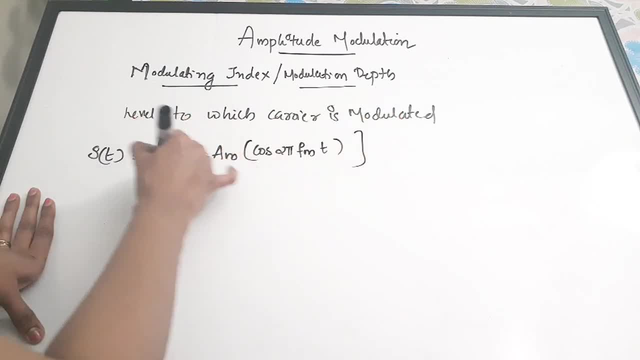 empresa which is connected to at vem into of lemma, into which we have as known as am modulated. well then, We are going to go to the next equation, which is that was done, a called. that is, this is the AM modulated waves equation. Now, from this equation, what I am going 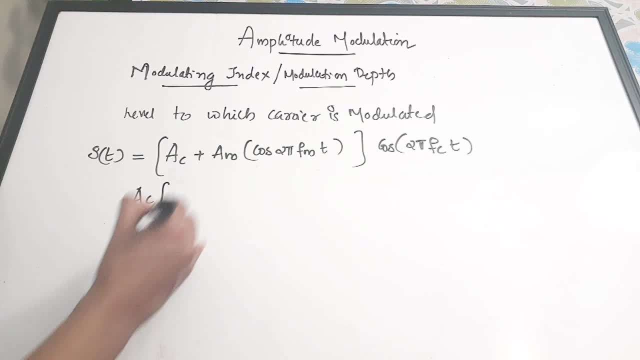 to do is I am going to take a AC as common. I hope you know that AC is the amplitude of the carrier wave, AM is the amplitude of the modulating signal or the information signal. FM is the frequency of your information signal. FC is the frequency of the carrier. So AC into I am going. 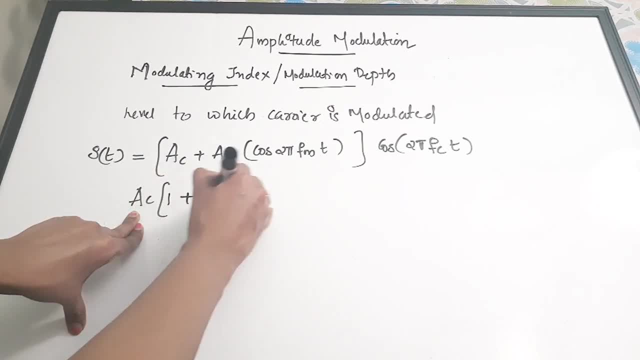 to take AC as common 1 plus AM by AC, cos 2 pi FMT into that is. I am just taking a AC outside, Okay, this into cos 2 pi FC of T. Okay, so here there is an AC outside and inside the bracket. 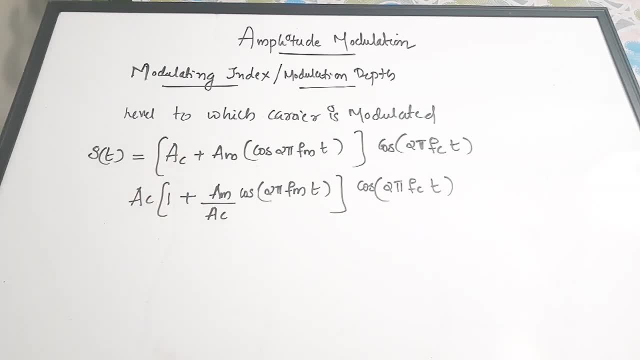 there is a AM by AC term, right. So this AM by AC, AC is called the modulation index, mu. So mu, that is, a modulation index, is equal to AM by AC. Now, AM, we know that it is the amplitude of the modulation, modulating signal or your information. 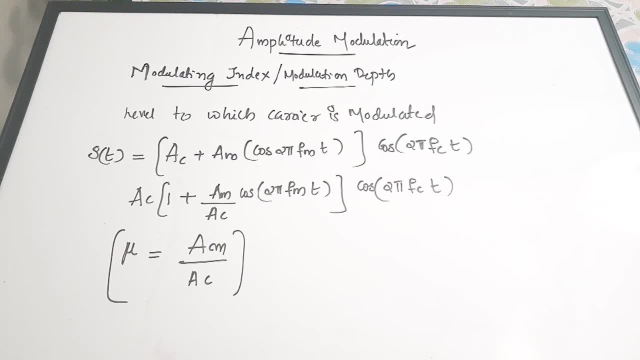 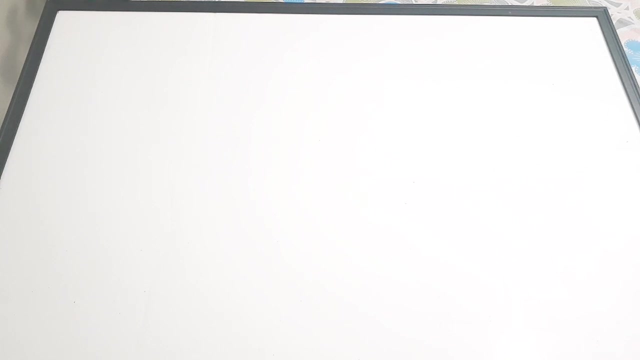 signal. AC is the amplitude of the carrier signal and its ratio. we call it as modulation index or modulating index. Okay, now there are some other terms, also in relation with the amplitude. Let us see that next. okay, Now consider that AM is the maximum amplitude of the modulated wave and AM is the maximum 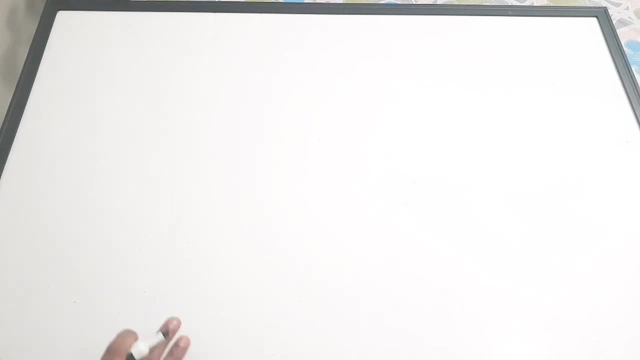 amplitude of the- sorry, minimum amplitude of the modulated wave. Okay, so we are going to define two terms: AM, which is the maximum amplitude of AM modulated wave, Okay, and we are going to define another term: AM minimum. We have already drawn that. 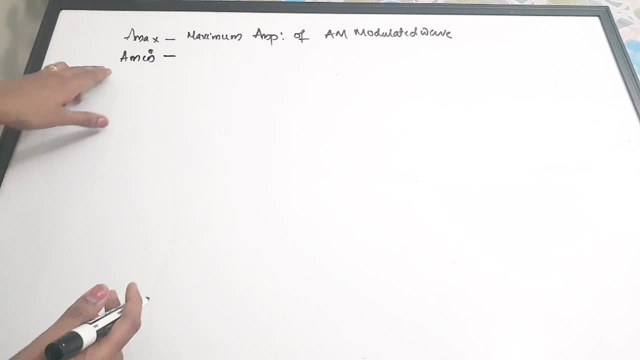 in the figure. Okay, maximum amplitude and the minimum amplitude, right. So AM is equal to the minimum amplitude of the AM modulated wave. Now, when we will get AM and when we will get AM. So AM actually we will be getting when Cos 2 pi fmt is equal to 1.. Okay, so we will get AMax when cos 2 pi fmt. 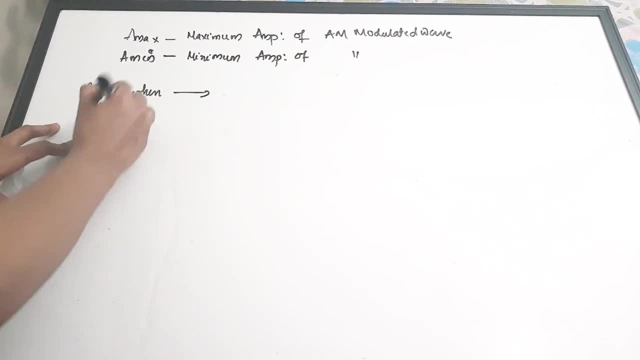 write it once again. Okay, so we will get AMax when cos 2, pi, fmt is equal to 1.. Okay, and the equation for AMax is equal to. AMax is equal to a c plus a m. okay, consider the. this is your equation number one. okay, so a max is the maximum. 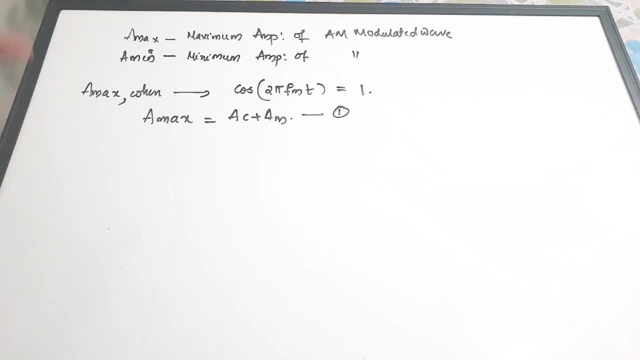 amplitude of your resultant a m modulated wave and the a max we are getting when cos pi- sorry, cos 2, pi, f, m, t is equal to 1 and the value of a max is equal to a c plus a m. okay, so in that equation- that is the equation- what is equation for your s of t? i'll tell you how the equation. 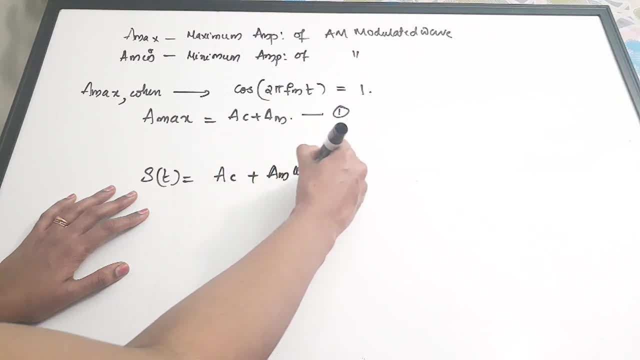 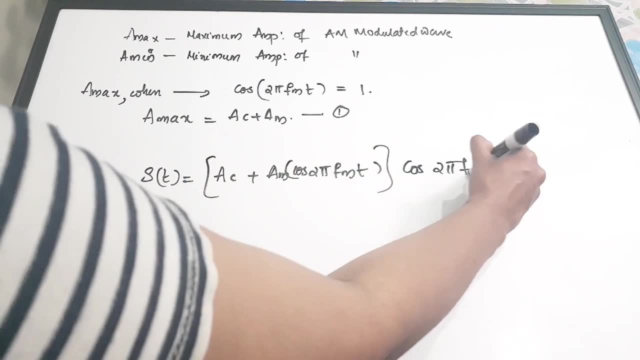 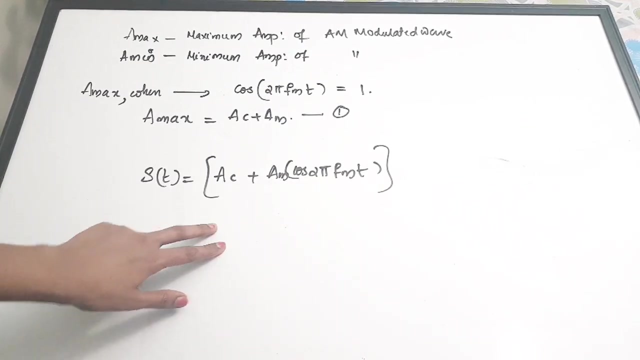 is coming a c plus a m, cos 2, pi f, m t. this is the equation right into cos 2, pi f c of t. now forget about the frequency or the phase part. we'll talk about only the amplitude part, this amplitude of the a- m modulated wave in the amplitude session, when we'll get the maximum. 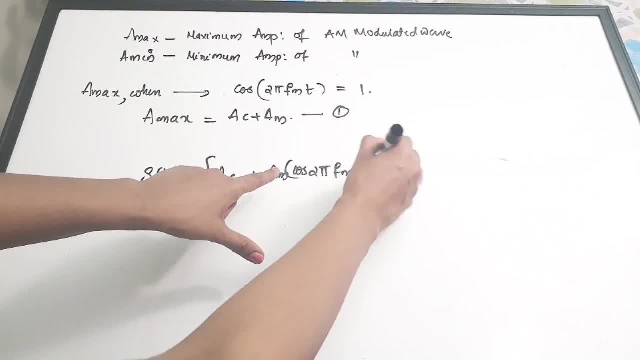 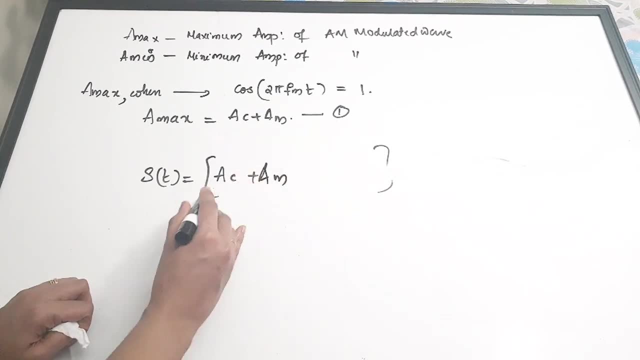 amplitude of the a m modulated wave. we'll get the maximum amplitude of the a m modulated amplitude is when this term, that is, cos 2, pi, fmt. when it is 1, we will get the maximum amplitude, which is nothing but ac plus af right, and we will call this amplitude. see, we are only talking about. 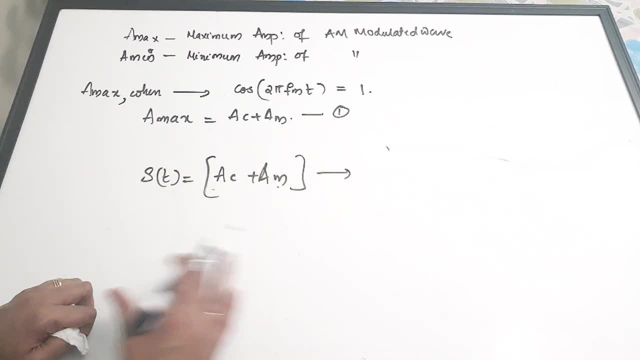 the amplitude part. we are not talking about the entire equation, only the amplitude part. we are taking. and in that amplitude part, when we will get the maximum amplitude. when cos 2, pi, fmt is equal to 1 right and the value is equal to ac plus am, we are calling it as amax. that's all okay, so that's. 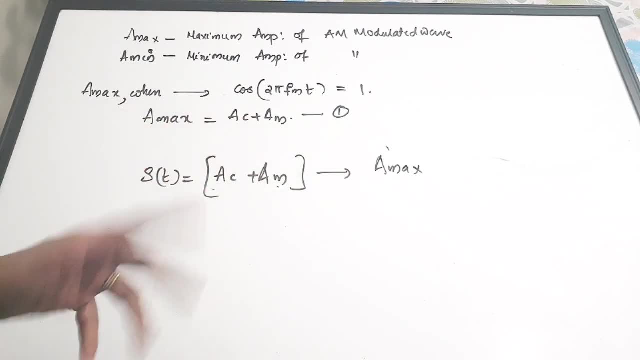 why i have written amax equal to ac plus am. i hope you understood how it is coming, okay next. next, we are going to define the second thing, which is the minimum amplitude. a minimum, so a minimum. we are getting, when cos 2, pi, fmt equal to minus 1. okay, so again. 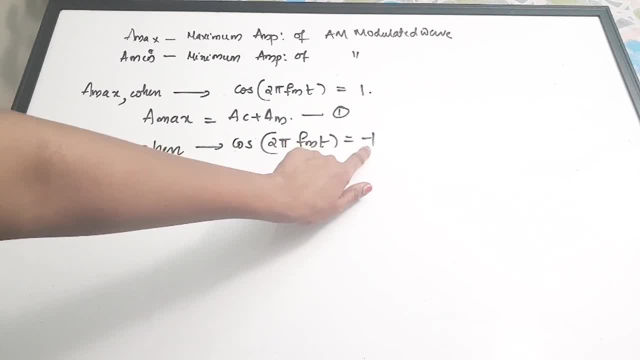 you will get the minimum amplitude. when the cos 2, pi, fmt is equal to minus 1, we will get the minimum amplitude and the value will be. i'm directly writing: a minimum is equal to ac minus am. okay, again, we are getting these equations from the am modulated wave equation. i'll show you that also. 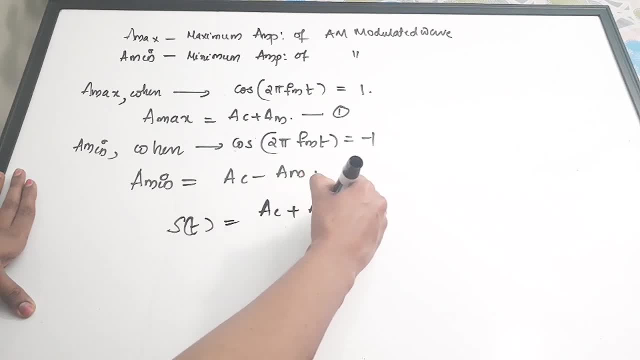 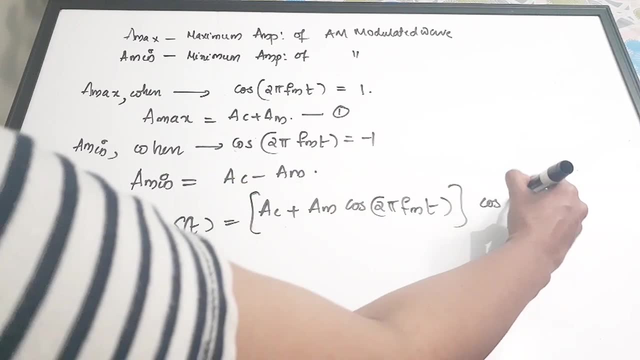 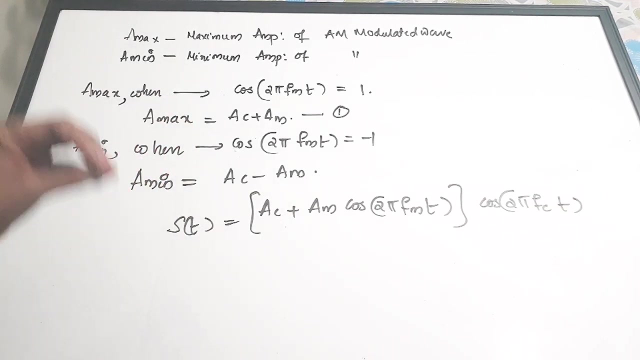 okay, s of t is equal to ac plus am cos 2 pi fmt into cos 2 pi fmt. so this is your equation, right? so this equation you should be knowing is by heart. okay, by the end of this video. anyway, you will study it by heart, don't worry. 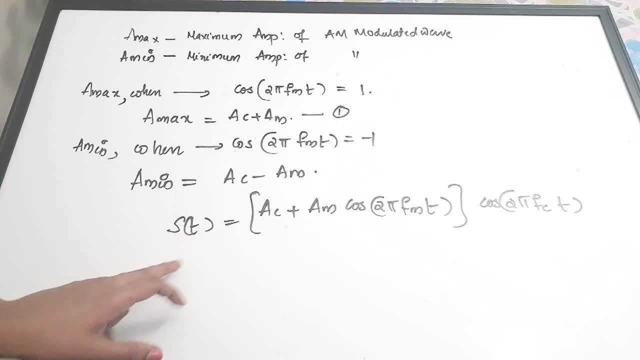 okay, so this is the resultant equation for your am modulated wave and in that wave, this is the amplitude part. this is the phase part. okay, so we will only consider the amplitude part now, because we are talking about the maximum and the minimum amplitudes, right, so when we will get the minimum? 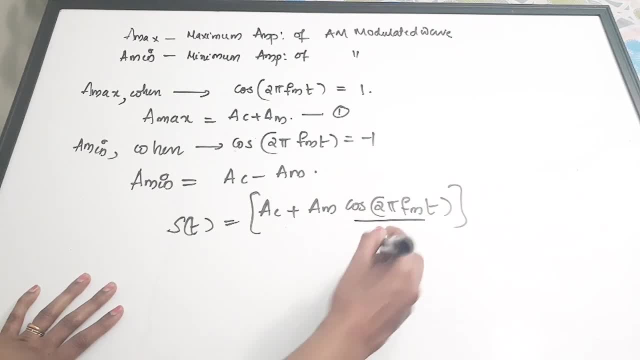 amplitude. when this term, this cosine term, when t is equal to minus 1, you will get the minimum amplitude and its value is equal to ac minus am. that we have called as a minimum right. So that also we have got. Now I am going to call. 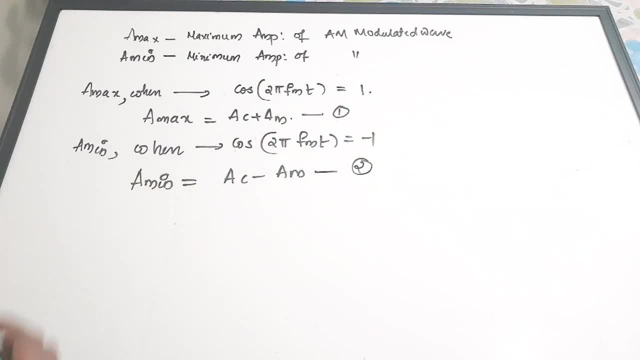 this as equation number 2.. Now, when I am going to so this is equation number 1, this is equation number 2.. 1 plus 2 you will get as a max plus a minimum, and that is equal to ac plus am. I am. 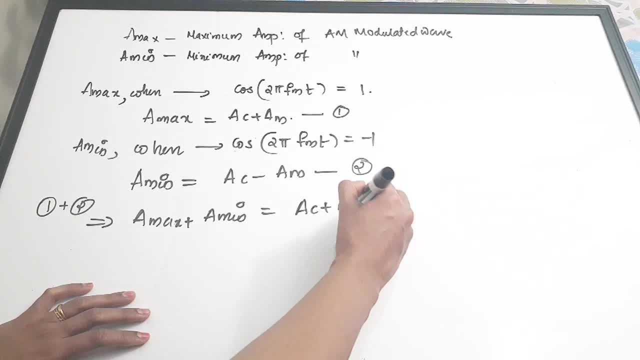 just adding equation 1 and 2. okay, ac plus am plus ac minus am. So this am am getting cancelled. you will get 2 ac right. So the equation number 2. you are getting is: if you add 1 and 2, a max plus a minimum is equal to 2ac. Similarly, if you 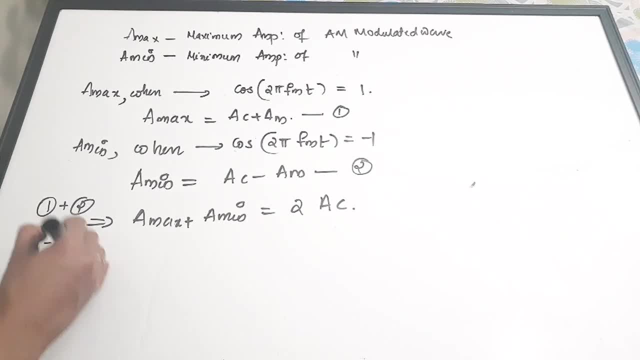 subtract 1 minus 2, what will you get? a max minus a min. you will be getting as ac plus am minus ac plus am. You will get as 2am right, 2am Okay. So you got two other equations. 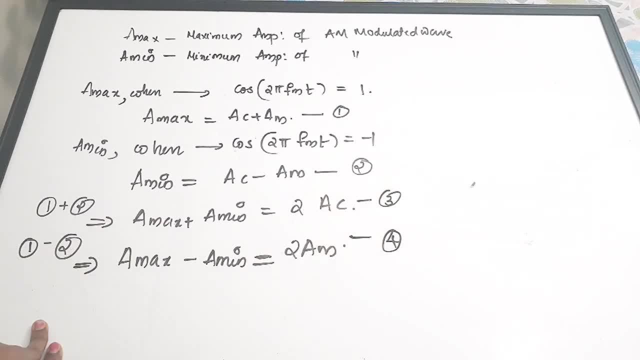 just call it as 3 and 4.. So the equation 3 is a max plus a minimum equal to 2ac, a max minus a minimum is equal to 2am, And from these two equations you can also write the expressions for AC and AM. Now, why we are actually discussing this is because you will 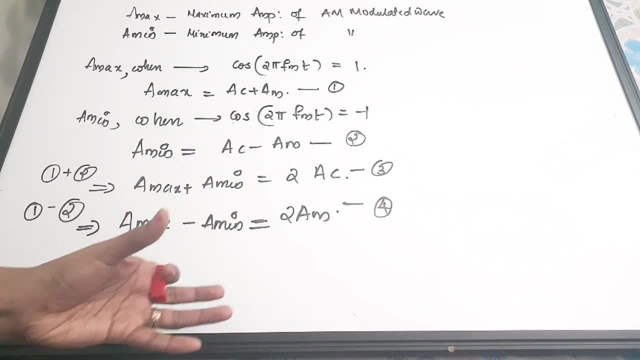 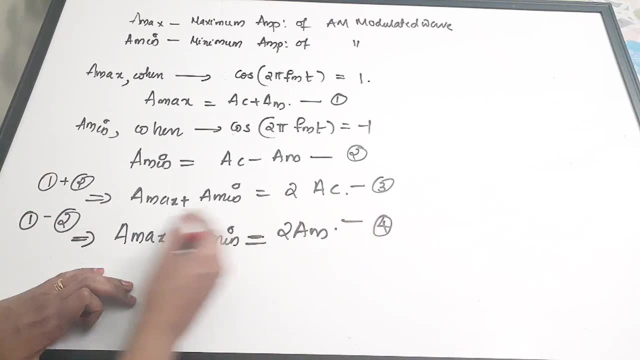 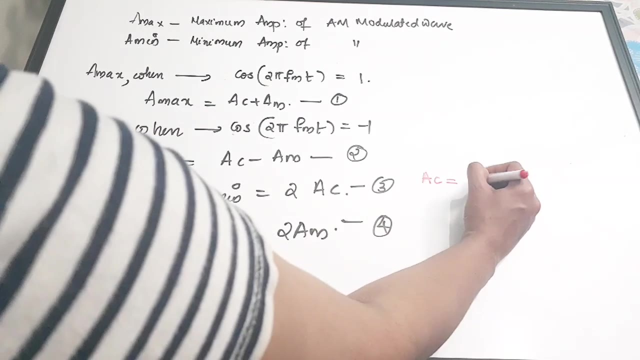 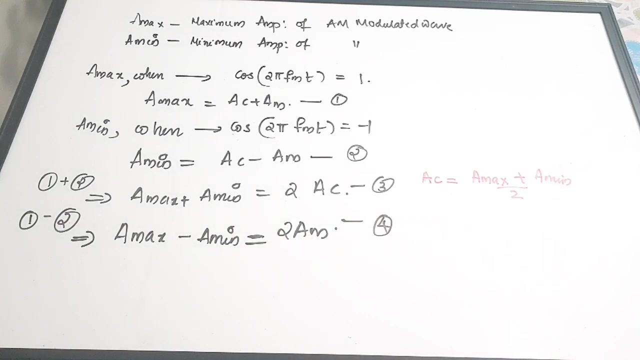 get use of these equations when you are especially preparing for competitive examination because you will get to do the numerical questions. So from the equation number 3 you can write: AC is equal to AMax plus AMin by 2.. So that is the equation you are getting. I will write. 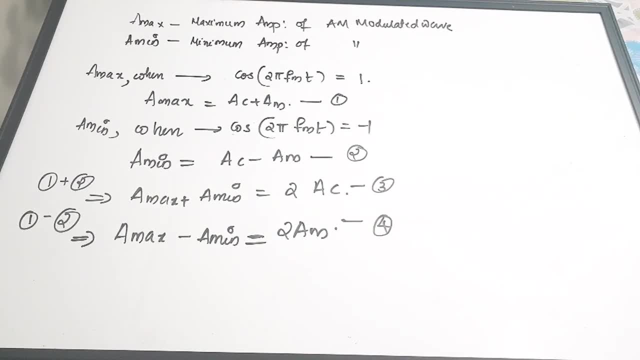 it once again. So the equation for AC you will get: AC is equal to AMax plus AMin by 2.. Similarly, from equation number 4 you will get: AM is equal to AMax minus AMin by 2.. Okay, These two equations are also very important. That is, you can write the amplitude of the 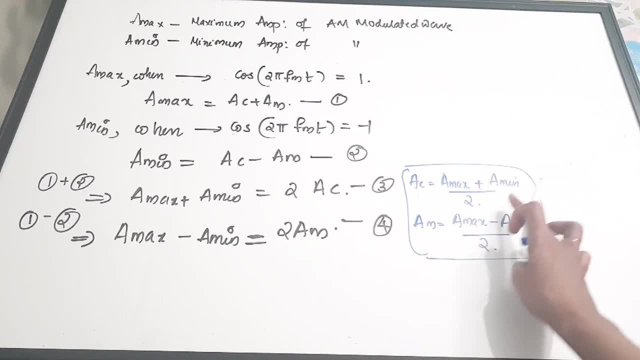 carrier wave and the modulating signal. if you know the maximum and the minimum amplitude of your AM modulated wave, That is, you can make use of these two expressions. And if you take the ratio of AC by AM, Now take the ratio of AC by AM or AM by AC, Okay, That is why that is what. 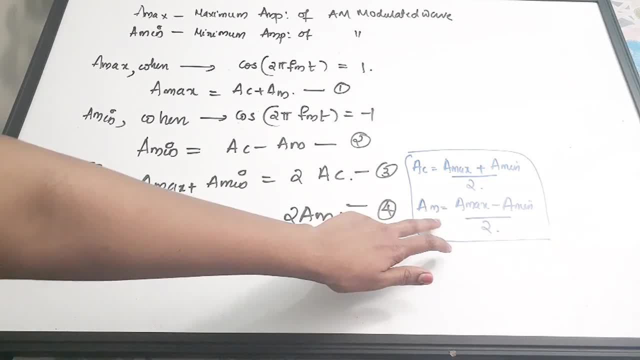 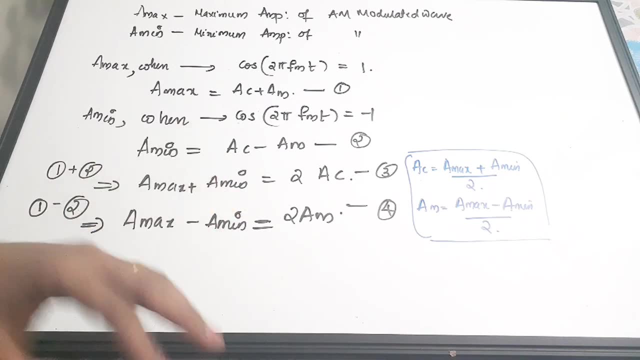 we are going to do here, That is, we are going to take the ratio of AM by AC and we know that AM by AC is nothing but the modulation index. So we are going to define the modulation index, or modulating index, in terms of the maximum and the minimum amplitudes. Okay, 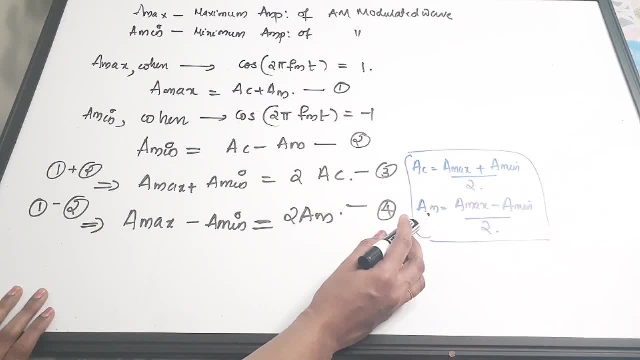 So these are the two equations for AM and AC. Now I am going to divide AM by AC. So AM by AC is equal to what will you get? AMax minus AMin by 2? and by 2 will get cancelled Right. So AMax. 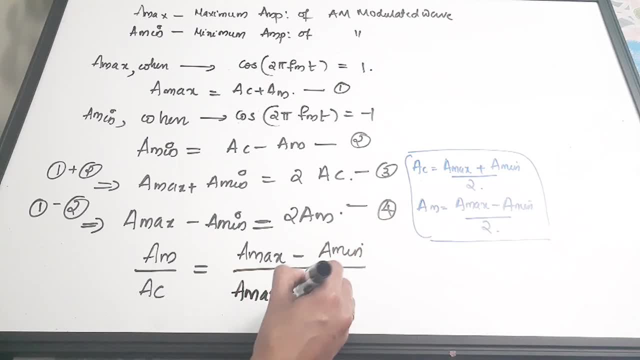 minus AMin by AMax plus AMin, Right? So this is the equation. So you can write this equation: Okay, expression for am by ac. and also we know that this is equal to mu, which is the modulation index or modulation depth. So here we have obtained the equation for modulation index in terms of the 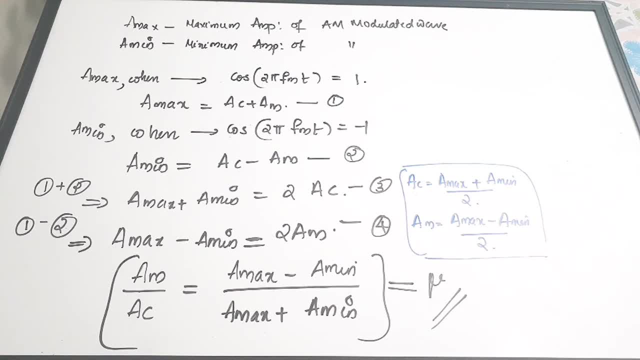 maximum and the minimum amplitudes of your am modulated wave. So first we have actually found the equation for the maximum and the minimum amplitudes and then we have taken the ratio of am by ac. So we know we have already defined am by ac is nothing but the modulation index. So if 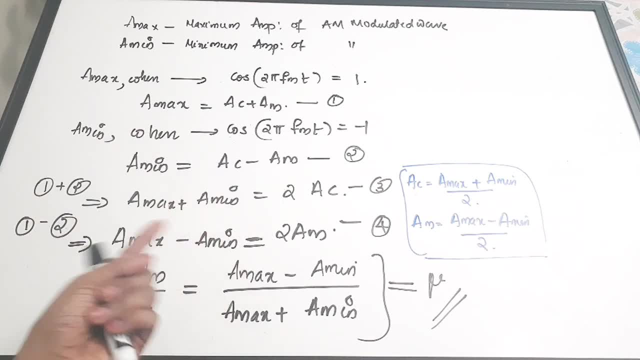 you take the ratio in terms of the maximum and the minimum amplitudes, you will get: am by ac is equal to amx minus amin by amx plus amin, So that is equal to the mu. So this equation is also very, very important, especially for community examinations. So we have discussed about 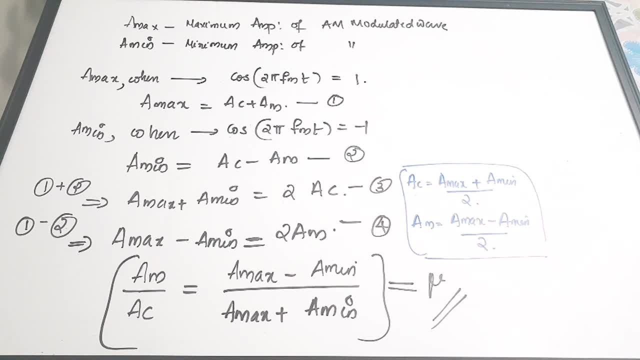 what is modulation index? and also we have defined term it in terms of the amplitudes, Now the value of mu. depending on the value of mu, whether it is greater than 1 or equal to 1 or less than 1, we say the wave by different names. Let us see that. 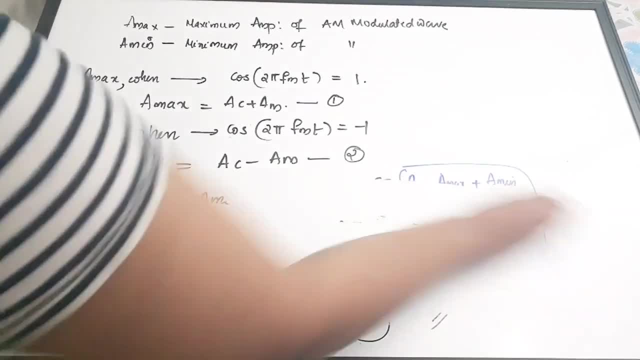 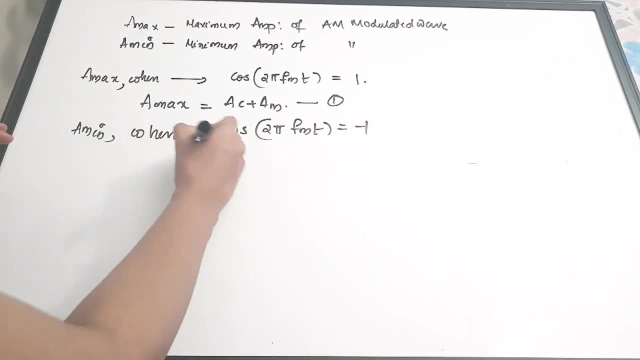 next. So, depending on the value of mu, you can define the wave, that is, a modulated wave, as various terms. When mu is less than 1, that is, if the modulation index mu or the modulation depth is less than 1, we say that the 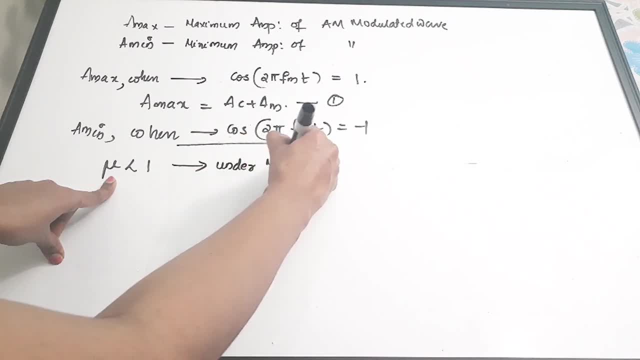 wave is a under modulated wave. That is the carrier wave. it is under modulated wave. When mu equal to 1, we say that the wave is critically modulated, Okay, And when mu is greater than 1, we say that is over modulated wave. So these are the three terms which we generally use to define the type. 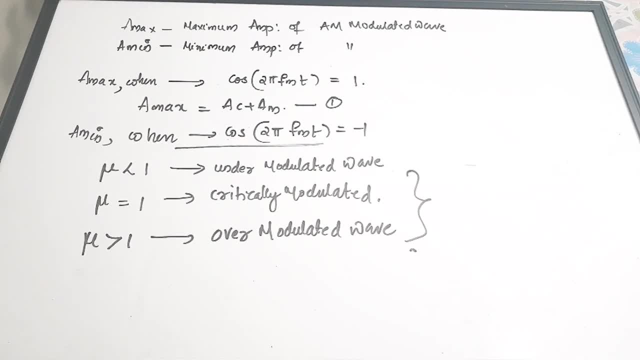 of modulation based on the modulating index. When mu is less than 1, we say that it is an under modulated wave. When it is equal to 1, it is critically modulated, and when it is greater than 1, we say that it is over modulated. okay, So these terms are also very important. Next, 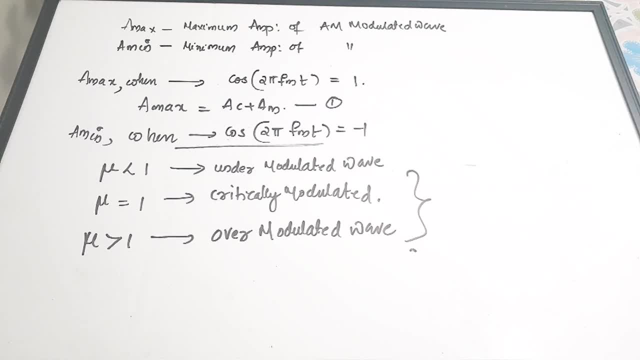 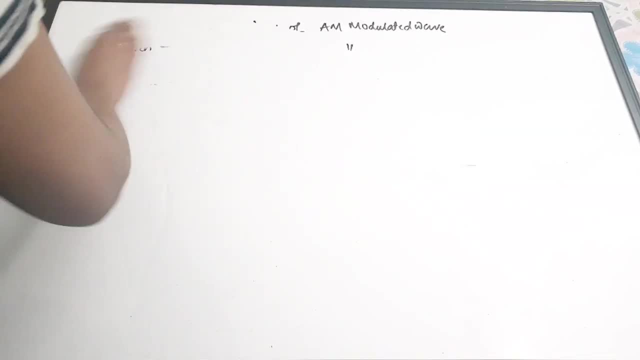 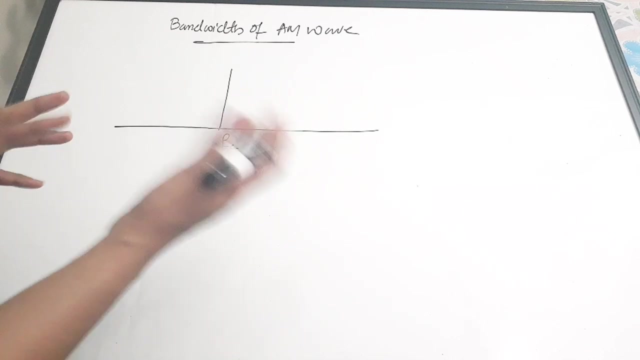 we are going to see the bandwidth of a AM wave. okay, The bandwidth expression is also very, very important, So the bandwidth of AM wave, okay. So, before defining the bandwidth, if you see the frequency of a AM modulated wave, there is a center fc, which is the carrier frequency, and on sides of 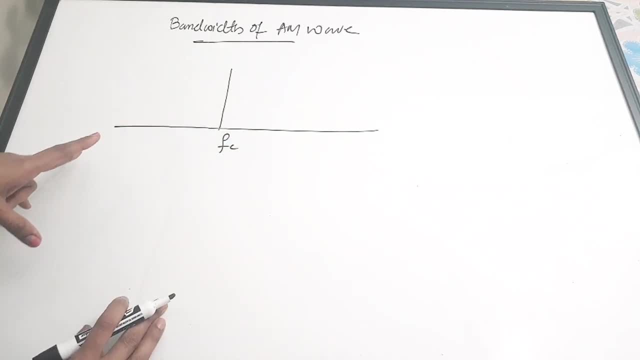 this center frequency. there is lower sideband and there is an upper sideband. okay, So this is the upper sideband, which is fc plus fm, and this is the lower sideband, which is fc minus fm. Now how we will get this: fc plus fm and fc minus fm. 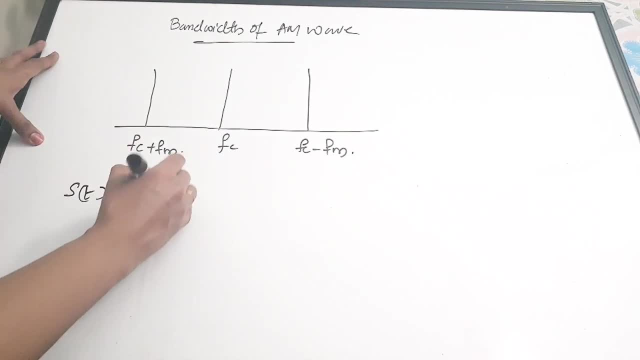 From this equation s of t itself. this equation is AC plus AM, cos 2 pi fm t into cos 2 pi fc t, right. So this is the equation for your AM modulated wave right Now. if we expand this, 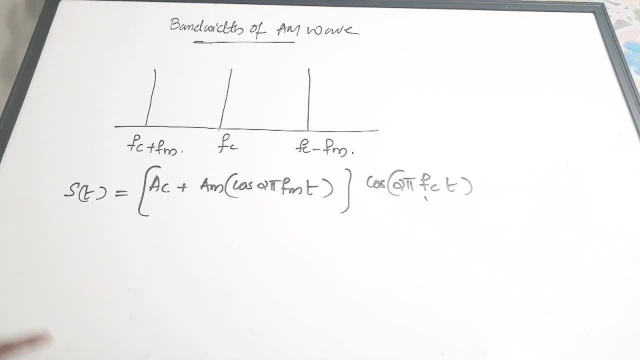 equation, you will get this Okay deliberately: fc plus fm. Next, if you expand this equation into fc plus fm, then is there anything per cent more, so frame rate of fc plus fm here, because of fc plus fm, in fact of it is the positiveoubl G х. 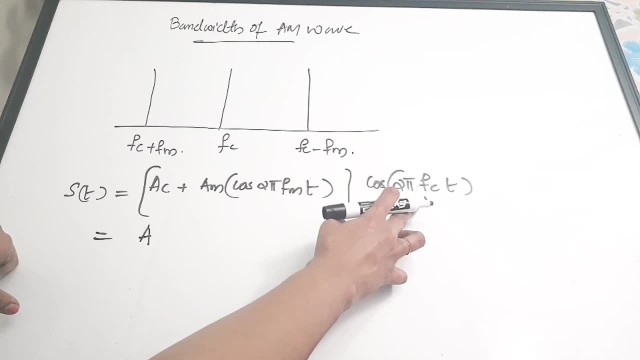 Then there is some manifestation which keeps us from ustedesi sense, in my opinion. So if we do the same fc and g goes way to the opposite direction. Next fc is not formas Kardamish. expand this cos inside this bracket. you will get ac, cos, 2, pi, cos, 2, pi, fct inside the bracket you. 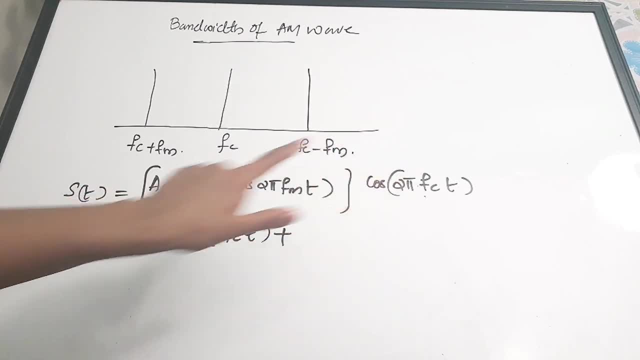 will be getting ac, cos 2, pi, fct. now if you take this cos and multiply with this cos, you have to apply in the cosine product equations, okay, and you will be getting the resultant like this: am by 2, cos, cos a, cos b. it will be. you have to write the resultant expression for cos a- cos b, okay. 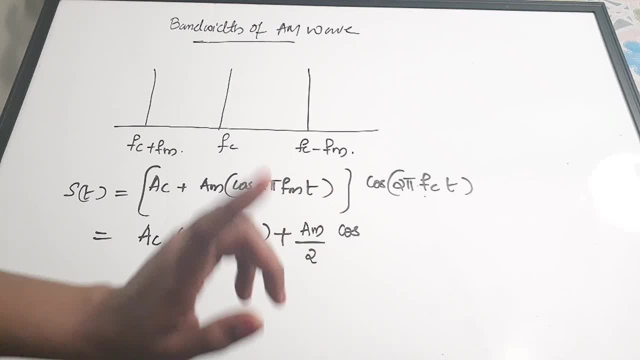 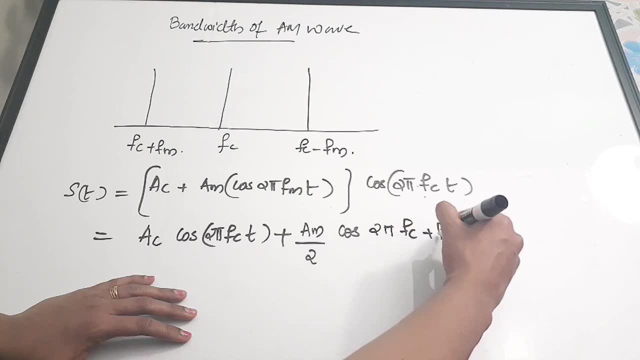 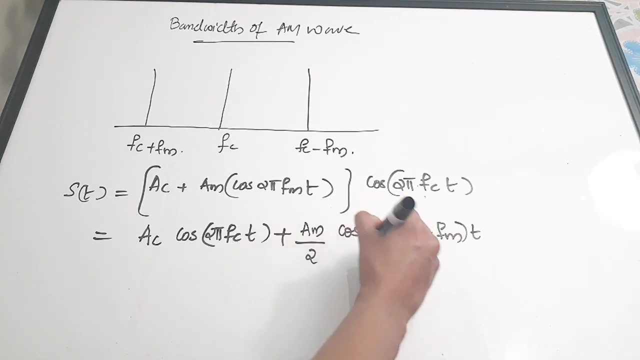 so it is 1 by 2 times, so am by 2. you will be getting, okay, i'm going to directly write the equation: cos 2 pi fc plus fmt. this is one term plus. the next term is again: am by 2: cos 2 pi fc minus fmt. okay, 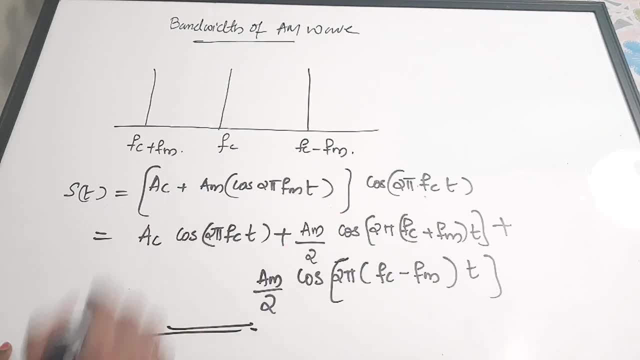 so this is: this will be the resultant expression in a more neat format. that is, you have taken this cos term inside the bracket. that is the only thing you have done, and you have also applied the equation for cos a, cos b. okay, so you'll be getting the equation like this, that is: 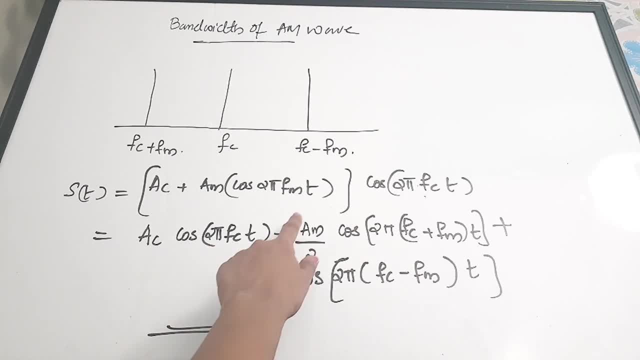 you have taken this söylenScript and you have taken this identification mixing equation. okay, is AC cos 2 pi, fct plus am by 2 cos 2 pi into fc, plus fm into t. So this is in the whole bracket of cosine plus am by 2 cos 2 pi, fc minus fm t. Okay, so there is a term. 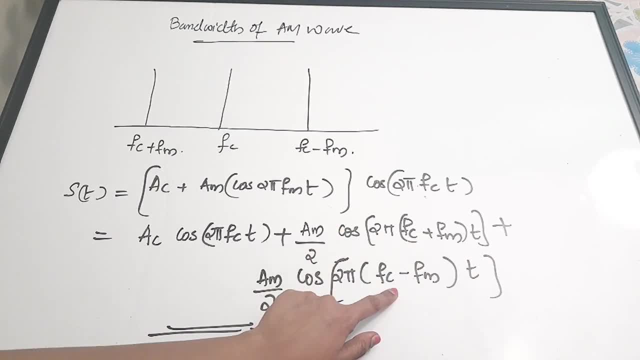 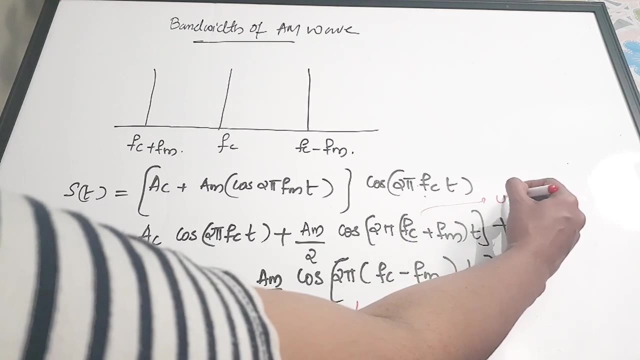 with fc plus fm, and there is another term with fc minus fm. So this fc minus fm, this term is called the lower sideband, or LSB, and this term with fc plus fm, it is the upper sideband, or USB. Now, from this equation we are actually drawing this spectrum, or this: 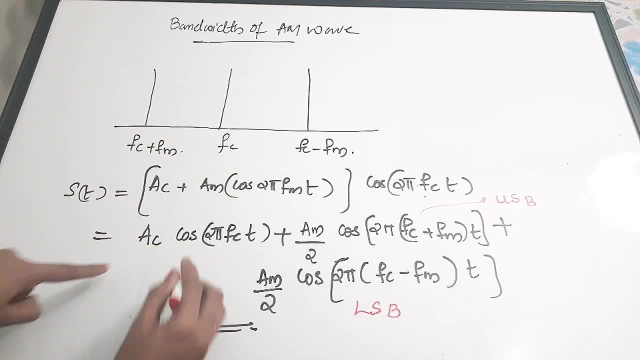 frequency diagram. So there is a sender fc which is corresponding to this term. Okay, so there is a sender fc which is corresponding to this term and there is a upper sideband which I have drawn here, which is fc plus fm. Okay, USB, and this is fc minus. 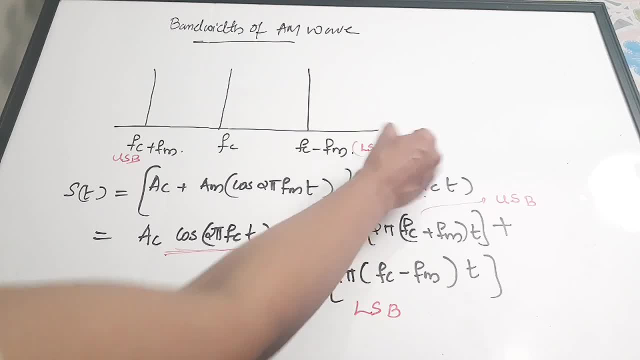 fm, which is LSB. Okay, so these are the three terms of the frequencies. Okay, now you can also write this: am by 2 in terms of the modulation index, That is, you can also write this as AC into mu also, We know that mu is equal. 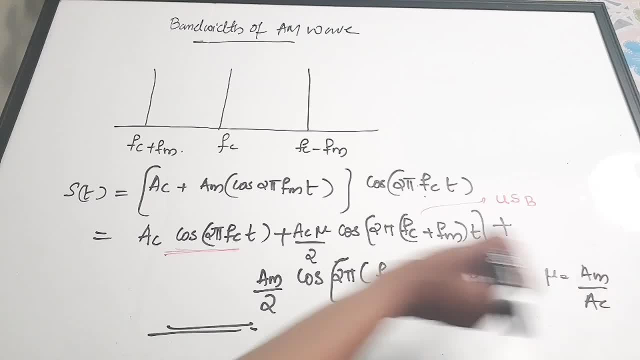 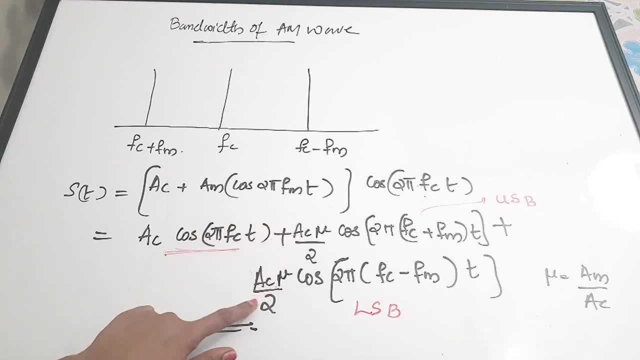 Okay, so now all the amplitude terms is having only the carrier amplitude. So here carrier amplitude into modulation index. Here also carrier amplitude into modulation index. Okay, so this is the total expression for your am modulated wallpaper. Okay, now keep. 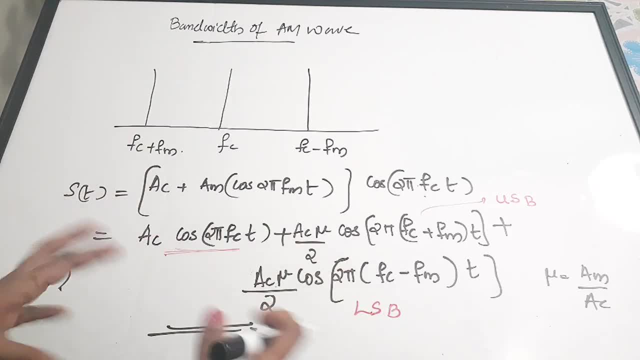 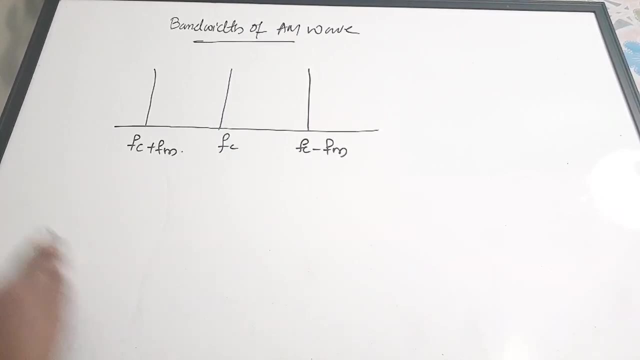 this thing in mind while finding the power equations which is negative to times l by equations. you again require it. okay, Now I am going to remove it as of now. okay, We just need the frequency terms for finding the bandwidth, okay. So these are the three. 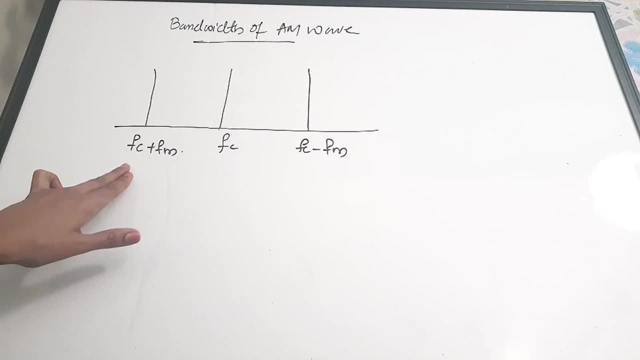 frequency components. that is the carrier frequency, that is the upper side band, that is a lower side band. Now we know that bandwidth is equal to f max minus f minimum. So for finding the total bandwidth we are going to take the difference between the maximum. 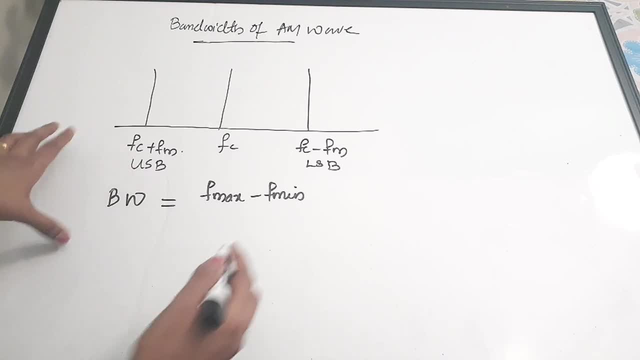 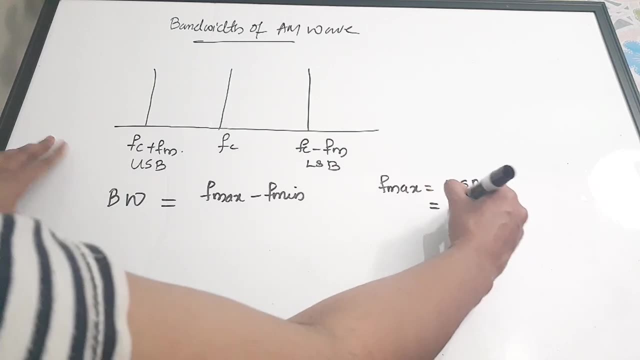 frequency and the minimum frequency. We know that here the maximum frequency, f max, is equal to actually our USB right and that is equal to fc plus fm right. Also, we are going to f minimum. it is actually the lower side band. The maximum frequency is this and this: 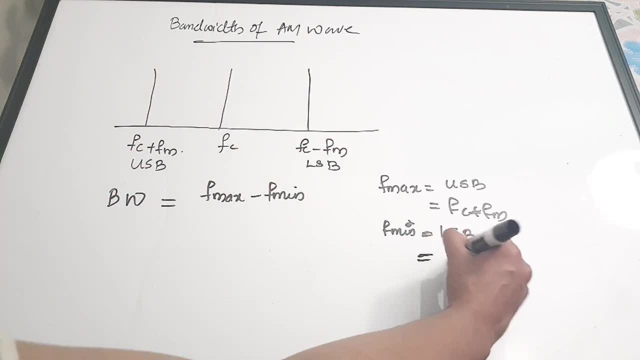 is the minimum frequency and it is equal to fc minus fm. So just substitute the values here. you will be getting the equation for bandwidth: fc plus fm minus fc plus fm. So you will be getting bandwidth is equal to 2 fm. okay, So this is the expression for 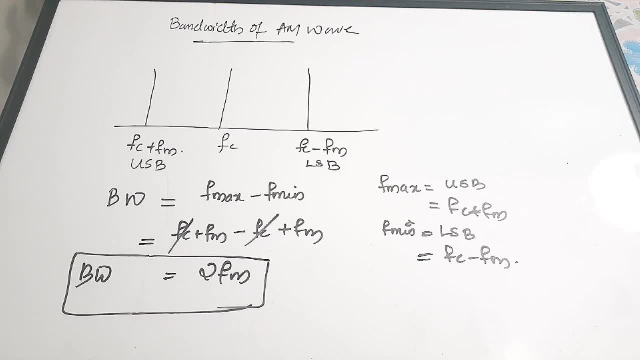 your bandwidth. So for a AM modulated wave, its bandwidth is equal to twice the modulating signal frequency. So in order to find the bandwidth of an AM wave, you do not require the carrier frequency, you only require your information signals frequency or your modulating signals frequency. 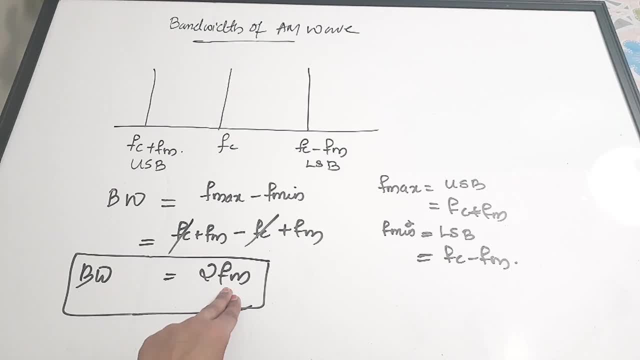 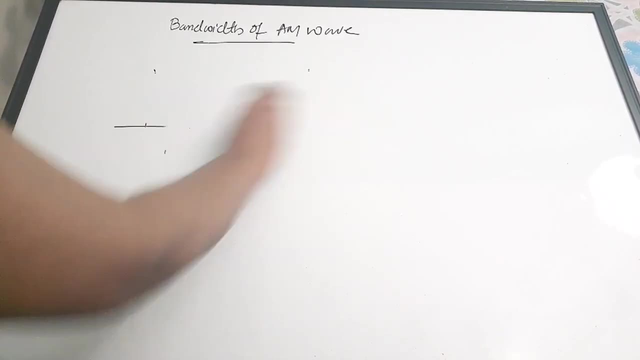 So the bandwidth is equal to twice the modulating signal frequency. okay, So that is all about the bandwidth. Next, we are going to see about the power equations, B-power equations. okay, So I am going to once more write the total equation for a. 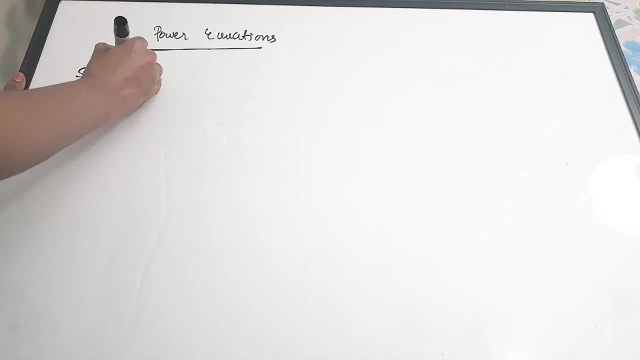 AM signal Directly. I will write: okay, ляются mä Brother. you write the power equations okay. So I am going to once more write the total equation for an AM signal Directly. I will write: okay. s of uiz equal to ac into fasb d, Sir Leroy, ok. 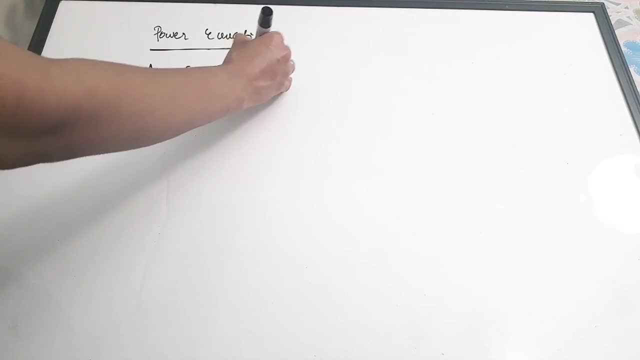 always tied by thelast bar and line stress greater than 2.5j X 1ils. months plus 23 hours kms by mGR V Excel �� cos 2 pi fct. This is one term and it is corresponding to the carrier. Okay. Then 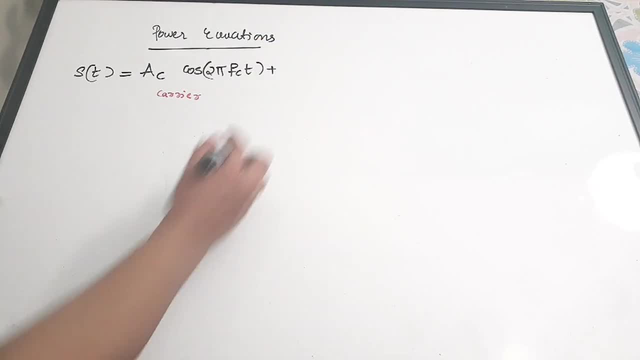 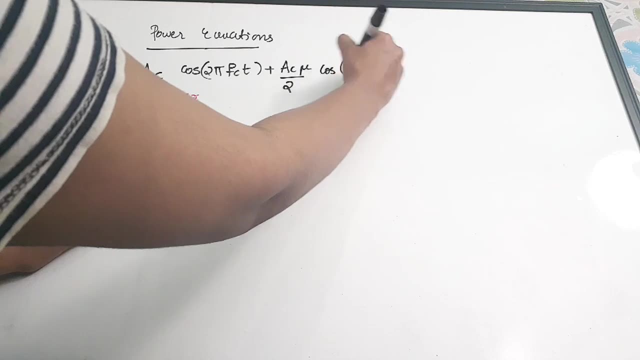 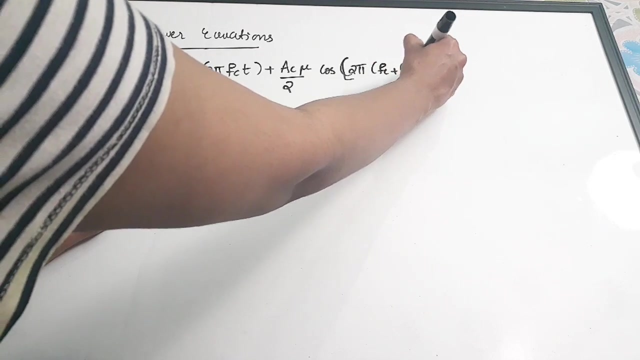 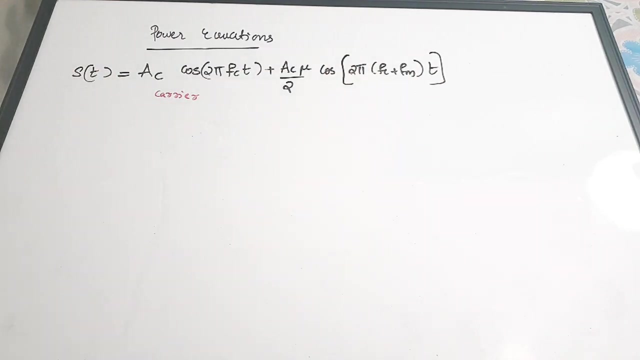 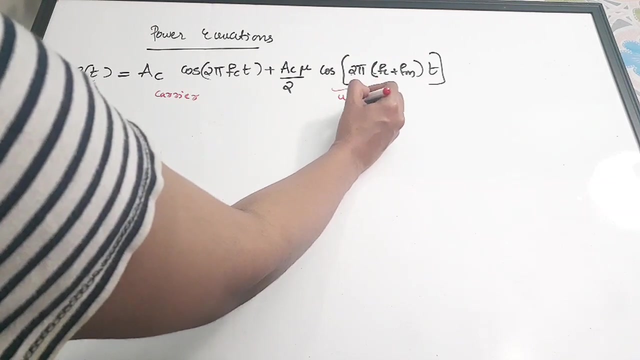 plus Ac into mu by 2 cos of 2 pi into fc plus fm into t. Okay, So that is Ac into mu by 2 cos of 2 pi into fc plus fm into t, And since it is fc plus fm it is corresponding to the USP, that is upper side band. Third, 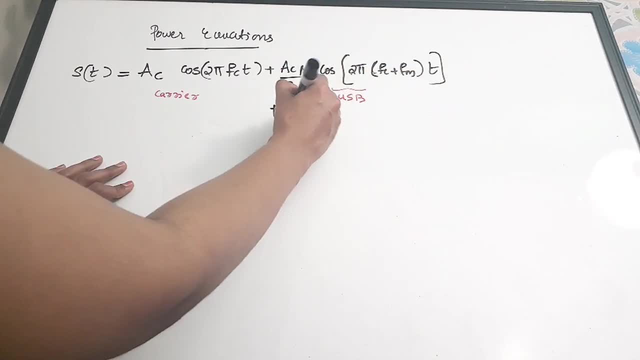 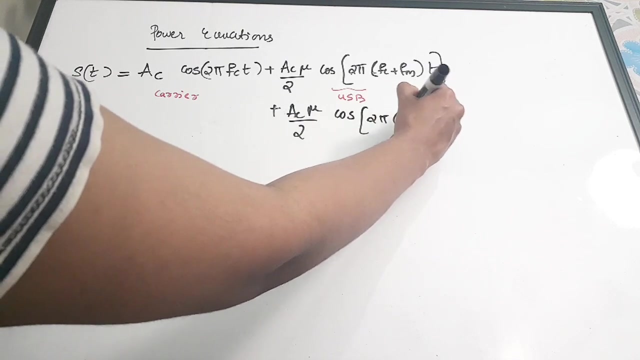 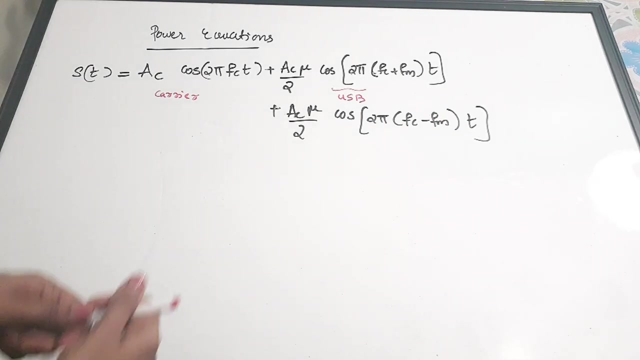 term I am going to write below: Okay, Here. So Ac into mu by 2, cos of 2, pi into fc, plus fm into t, Right? So the third term is corresponding to the lower side band, Right? So if you examine, 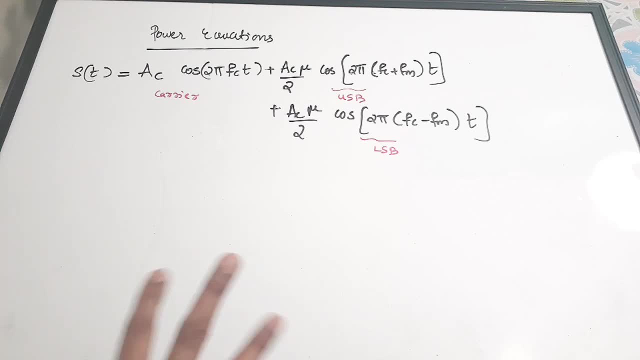 the total equation for an AM modulated wave, there are three terms: One term corresponding to the carrier. second term corresponding to the upper side band. third term corresponding to the lower side band. Also, you should be understanding that there are three terms, or 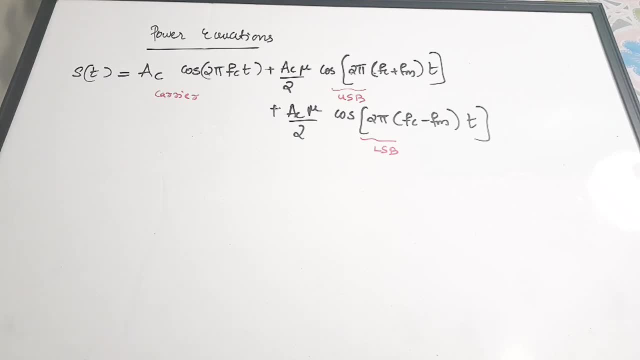 three side, yeah, three parts of a AM modulated wave. So you should be understanding that higher modulated wave. Why? Because while we study the wherenie various variations of AM, that is, one side band suppressed carrier or double side band suppressed carrier or 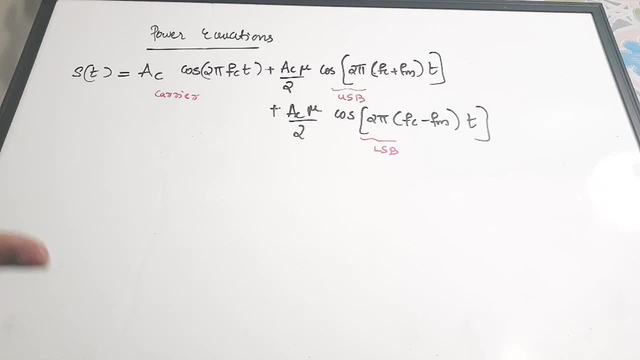 single side band: suppressed carrier. there are lot of variations of the AM. I hope you have heard of those things. Okay, While studying those, you should be knowing that the initial wave, or the initial AM modulated wave or the basic one, is having actually a carrier part. 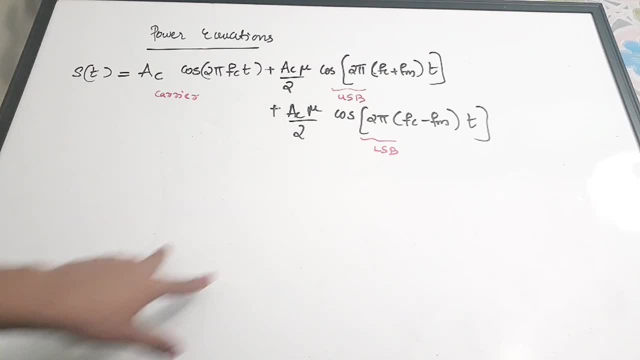 or the carrier Đâyahin being carrying over time. you should be knowing that the initial or the initial AM modulated wave, the basic one is having actually a carrier part or the carrier term, an upper side band and a lower side band And the other variations of this. 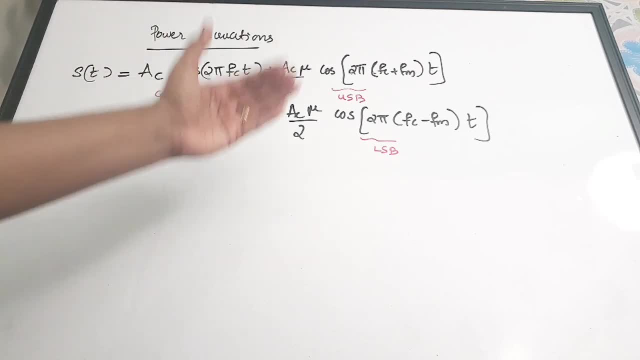 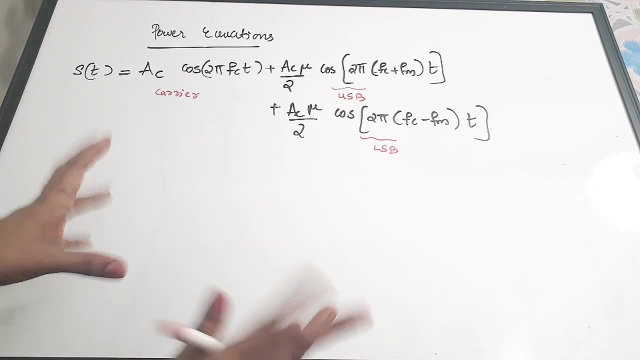 AM we actually produced by either avoiding one of the terms or two terms likewise. So the basic AM wave is having three terms. One is a carrier, upper side band and a lower side band. Now here we are talking about actually the power equations, So we can write that: 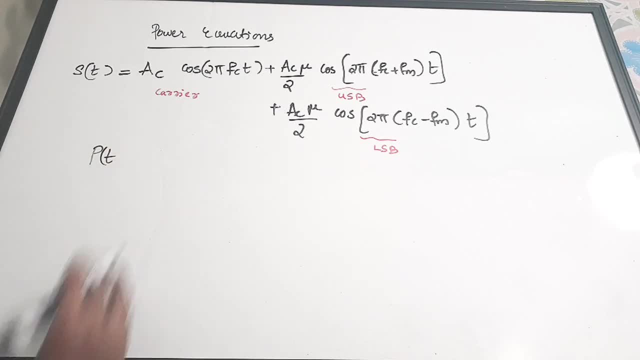 as there are three terms: the total power PT. if you call the total power PT, it is constituted by the carrier power plus upper side band power plus the lower side band power. Okay, So these three terms constitute to the total power Right And the equation for the 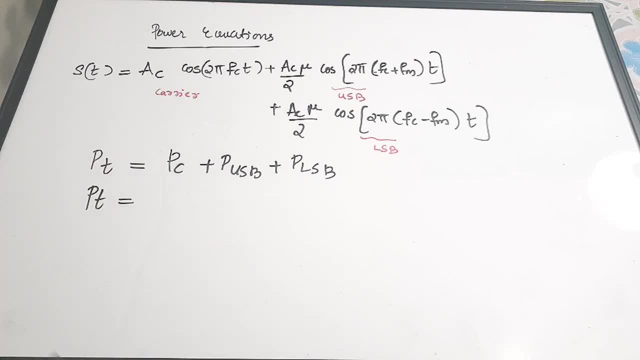 total power you are actually getting by taking the Okay Ratio of the RMS voltage square by resistance. Okay, We know that P is equal to V square by R. There are other terms also, but we can use the equation: P is equal to V square by. 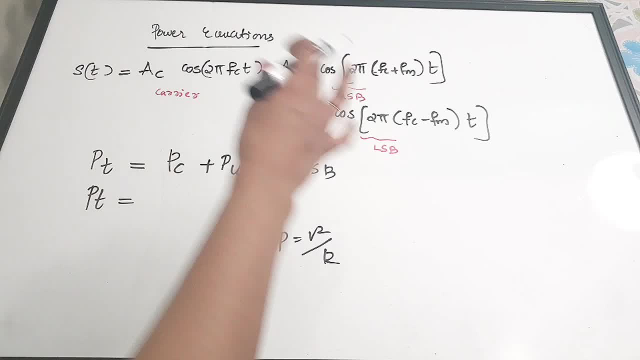 R. So for finding the power, we are actually taking the RMS value of this signal's voltage and dividing it with the resistance. Okay, Now here I am going to directly write the equation, because we do not actually require the derivation or anything. So PT is equal. 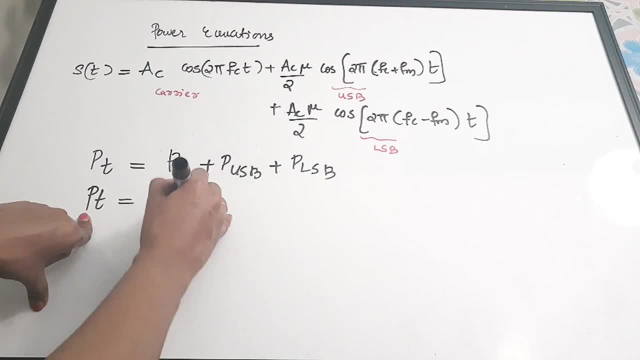 to this equation is very, very, very important: Pc into 1 plus mu square by 2.. So we have already said what is a mu. Mu is a modulation index. So the total power we are getting if you take the product of carrier power into 1 plus. 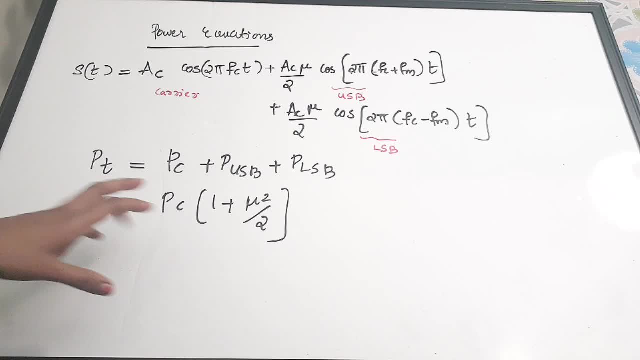 mu square by 2.. Okay, And also if you substitute this term here, so this is equation 1, I am going to call it as equation number 2.. Substitute mu: mu is equal to mu and the value The power. 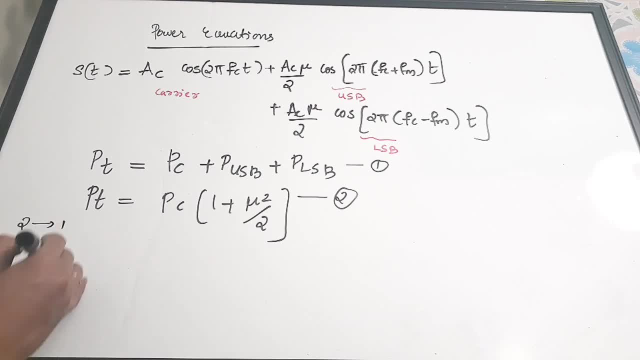 of the carrier. the total power we are getting is counted at the product of carrier power. Okay, And also if you substitute this term here. so this is equation 1, I am going to 2 in 1.. You will be getting PC into 1 plus mu. square by 2 is equal to PC plus PUSB plus PLSB. 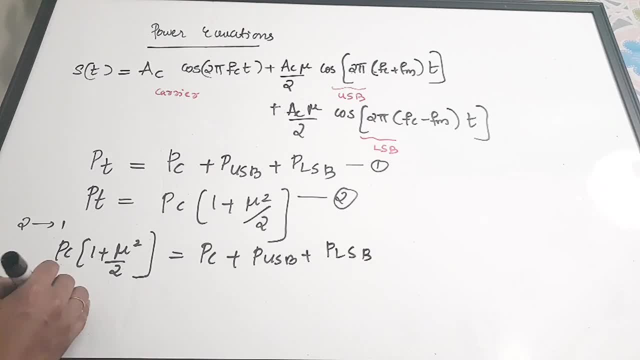 Right Open this bracket. PC plus PC into mu square by 2 is equal to PC plus PUSB plus PLSB. Okay, You can cancel out these two PC terms. Okay, Now this equation is also very, very important. 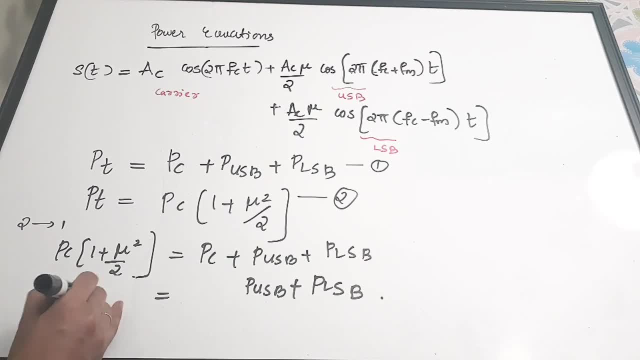 I will rewrite it once again. Okay, In a neat form: PC into mu square by 2.. Okay, So the total power constituted by the two sidebands, that is, power of upper sideband plus power of lower sideband, is equal to PC. 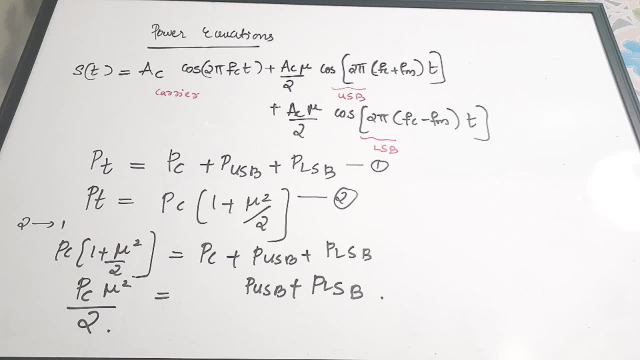 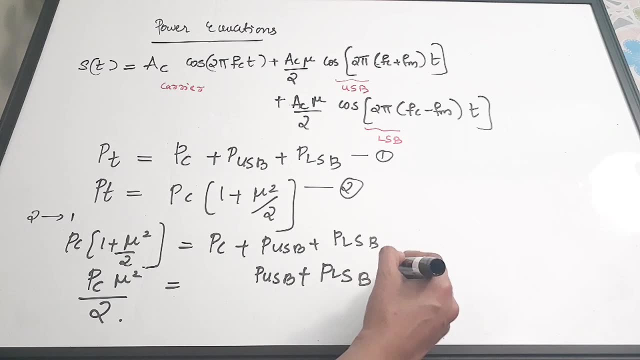 PC into mu square by 2.. This equation is also very, very important because a lot of numerical questions you can face, especially in competitive examinations, using this equation also Okay. So please note this equation also. The total power constituted by two sidebands. 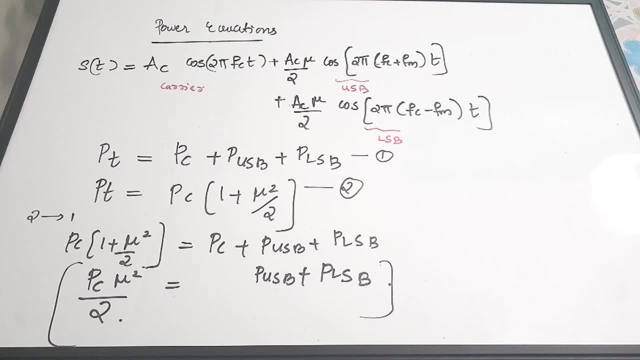 together. Now if you want to find the power constituted by the individual, by any individual sideband generally, we will take that both the sideband constituted power is equal and we divide it by This equation by 2.. Okay, That is, we take PLSB is equal to PUSB is equal to this total. 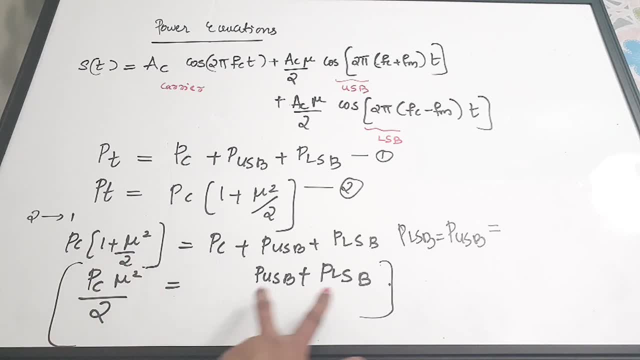 power. This total power is actually constituted by the sum of these two powers. So if you want to find individually the powers, then we divide this term by 2.. That is the general equation we are using. Okay, PC into mu square by 4.. Okay, This is the equation we generally 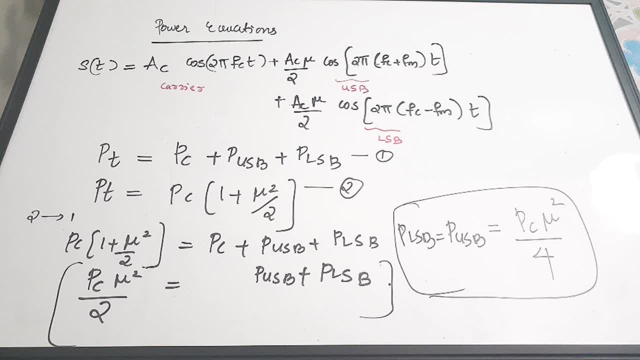 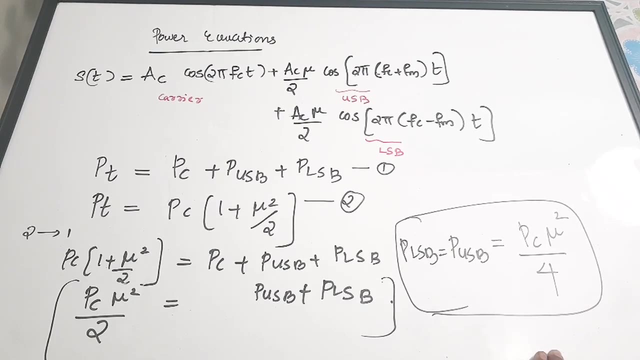 using. We are using the same equations for some other variant equation or different equations also, But generally we use this equation for finding the powers of the either of the sidebands. Okay, PC into mu square by 4.. Okay, I hope it is clear. So these are the important power. 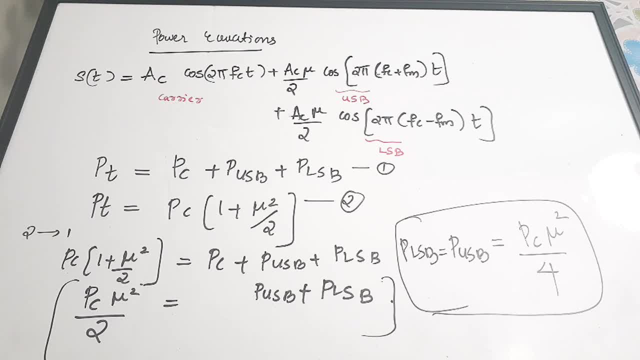 equations for an AM modulation. Okay, So in this video we have actually discussed about what is AM, what is the modulation? what type of modulation is happening there? how is its waveform looking like? What is the bandwidth equation? what is the modulation index? how can we define modulation? 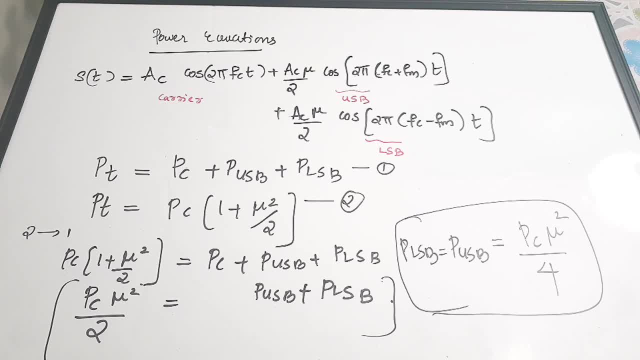 index in terms of the maximum and the minimum amplitudes. Also, we have seen the bandwidth equations and the power equations. Okay, So this video is a total revision of a amplitude modulation topic. I am really hoping that you understood the topic. So if you study, 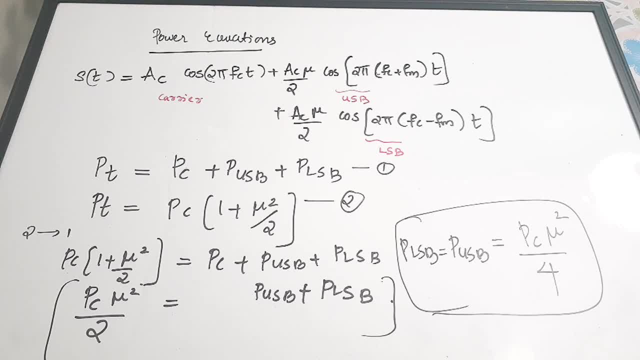 these most important equations. it will be very useful if you are preparing for some competitive examinations. Okay, So let us see what is the bandwidth equation. So let us see what is the amplitude equation. Okay, So, if you study these most important equations, it will be very useful. 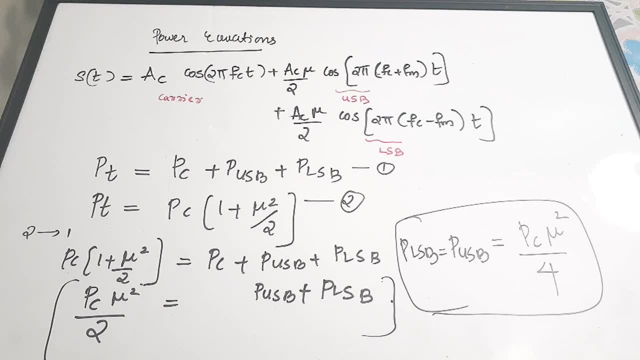 if you study these most important equations. So let us see what is the amplitude equation. So let us see what is the amplitude equation. So please do share it with your friends, Okay, If you are preparing for some competitions or your friends is preparing, and also if 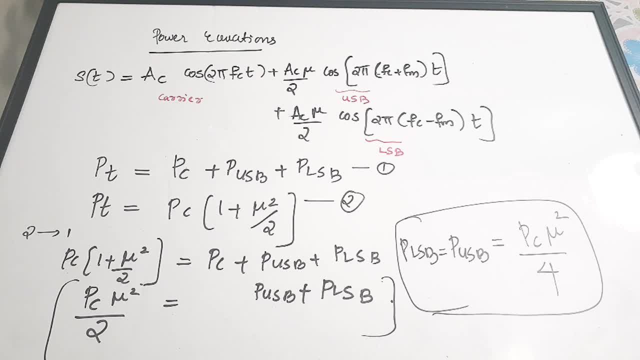 you want more videos, please do subscribe to the channel. Thanks for watching and keep on watching.